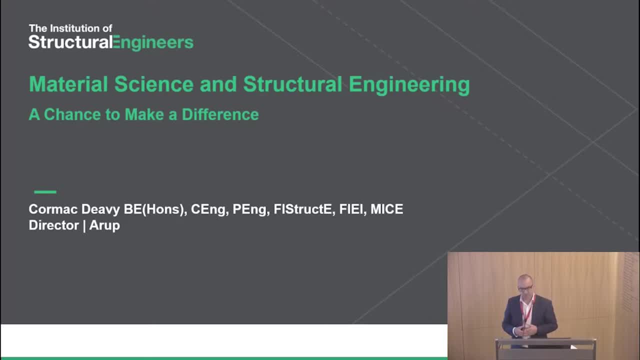 dive into that, but with a digital and computational design overlay about a particular project. And the third part is about looking to the future a little bit. So let's see if I have more luck with the clicker than Elizabeth. So this is the start. 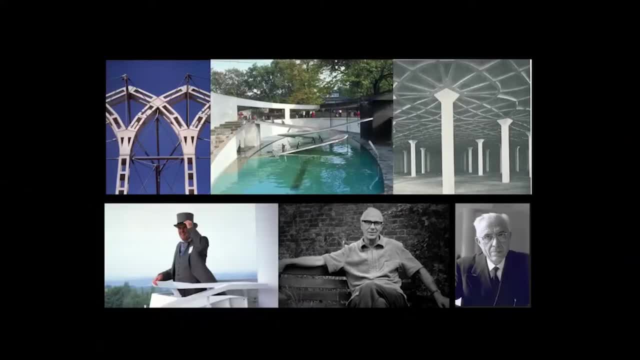 It's about exploring materials in my early career. So I suppose early on in my career and through well starting through my education in early career, I was very excited and I suppose influenced by the work of the three gentlemen along the bottom, working from right to left: Pierre-Luigi Nervet, then Ove Nyquist-Arp and Peter Rice. 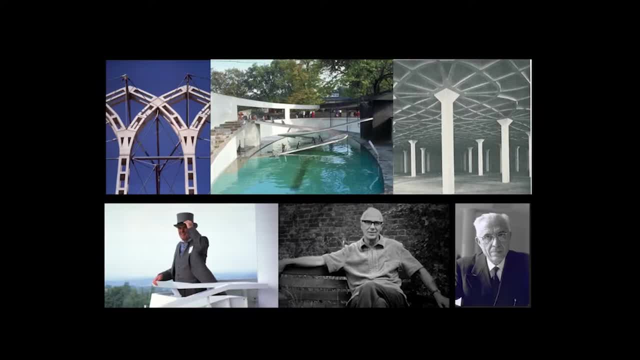 the two on the right-hand side I noticed on the board are gold medal recipients And what I was really interested about their work is that the approach that they took to structural engineering And Nervet very much was about understanding the flow of forces in structures and then 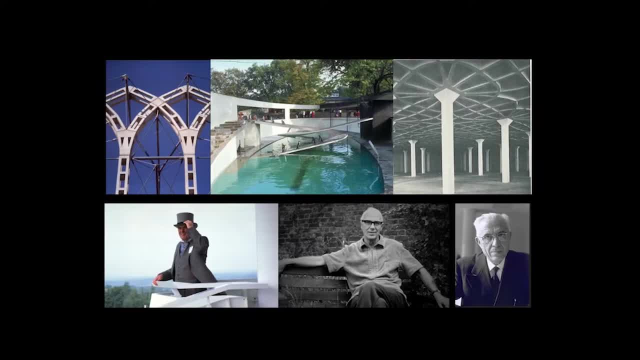 tried to optimize the use of materials, where you put the material where it was needed, based on the flow of forces. Ove then took things a little bit further and he was really looking at buildability, collaboration, constructability and again about exploring. you know different ways. 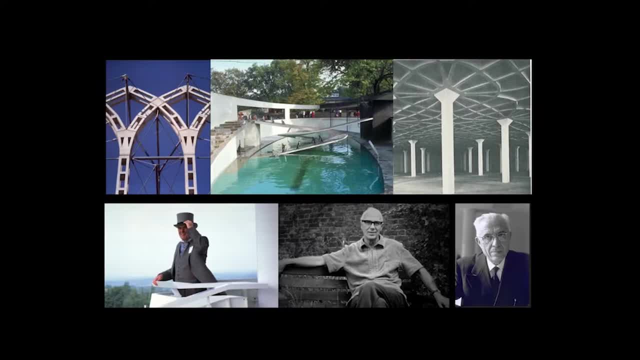 to build. And then Peter, an absolute genius. but what he did was start looking at alternative materials, but also different computational and analytical techniques, so that we could optimize and get the best value out of the materials that we use. And I think for me, what these did was it showed that you really needed to have a fundamental 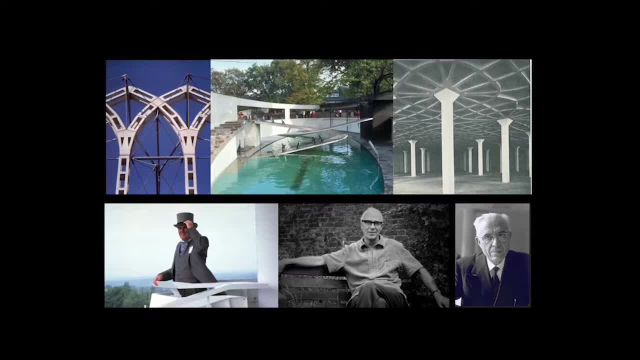 understanding of the science of the material and the physics of the material and it really drove a first principles approach to design. And what I got from that Personally is it gives you a lot of freedom when you do it from first principles, going beyond code. 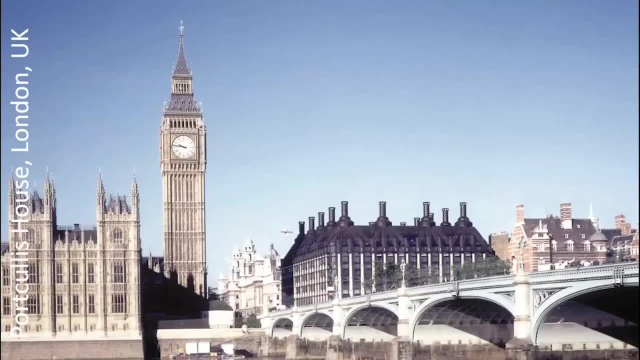 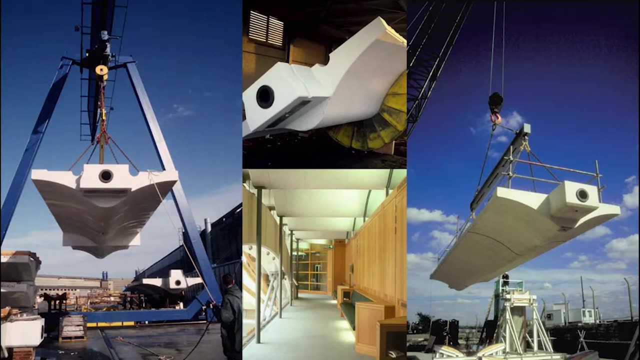 It gives you freedom to explore new avenues. So I'm going to talk a little bit about one of my projects which where I did that in different aspects of exploring materials and design. that's Portcullis House in London. So the first part of this was the concrete floor slabs and you might think, well, how is? 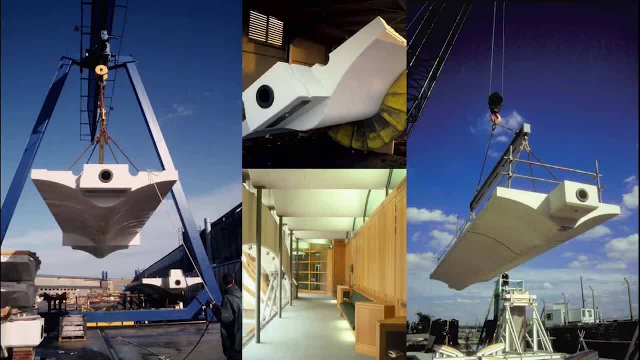 that a new material, But a lot of the work is about how you use existing materials in kind of new and innovative ways. But what we looked at here was we had a grid of 13.6 meters clear span and, working with the architect, Michael Hopkins, who was also influenced by Nervi, he wanted to understand. 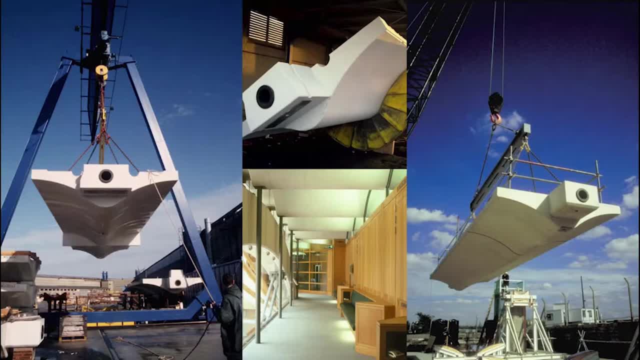 and try and create, use the minimum amount of material to get from A to B spanning 13.6 meters. So we looked at how we would do that and rather than kind of doing, I suppose, a traditional approach to design where you might design a slab and then optimize it and pull out a 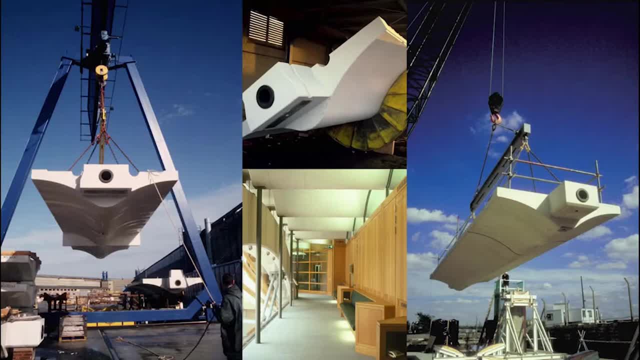 few millimeters here and there and reduce the amount of rebar. we looked at it quite differently. We said: what are all the other things that the concrete needs to do and what is the minimum amount to achieve those particular goals? So when we looked at fire separation between floors, acoustic separation between floors, 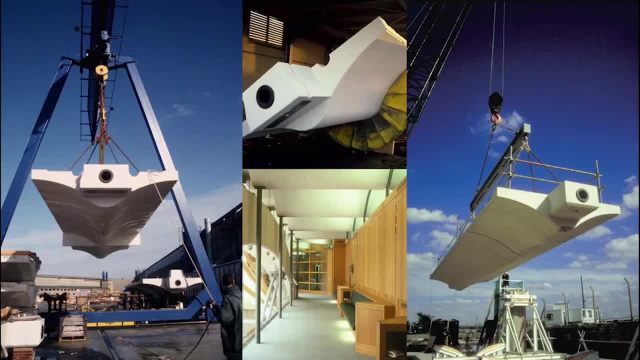 and everything else we came up with. the dimension of 125 millimeters was needed to achieve that. So then we said: how can we get 125 millimeters of concrete to span 13.6 meters? and that's what we did. So, even though this looks quite big, what we did was we created the form to create a lever. 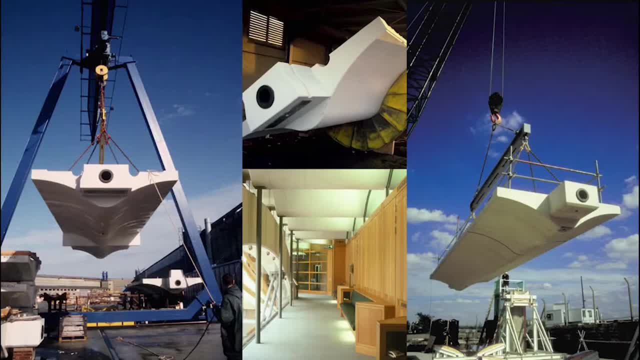 arm between the tension and compression slanges. that allows it to span 13.6 meters. 13.6 meters with 125 mil of concrete, and this is what we did. but actually to achieve these precast units was really working closely with the manufacturers and and with the contractors. 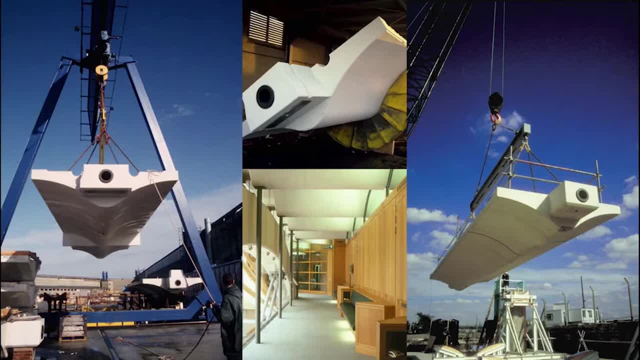 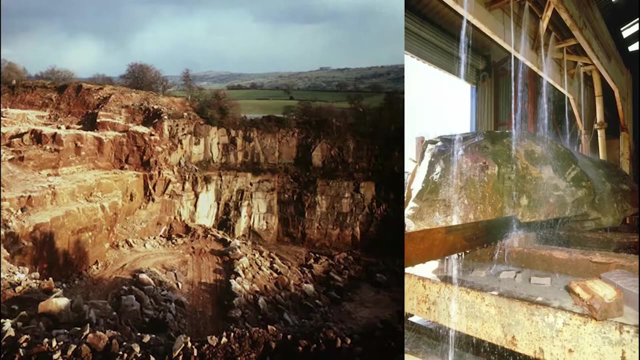 to really understand, use a construction-led approach to the implementation of the precast, so that to me was really understanding the construction process, the material itself and um and the on-site uh construction- another part of the, the project that we looked at, and this was: we were in a world heritage site for this particular building. we had to replicate. 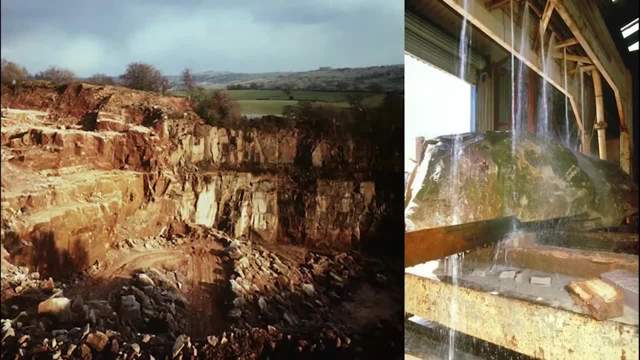 the, the materials used in the surrounding area and a lot of that was was natural stone and hopkins as an architect. they're very true to the materials. they don't. what you see is what you get. they really don't kind of hide things with with, with cladding and finishes and everything. 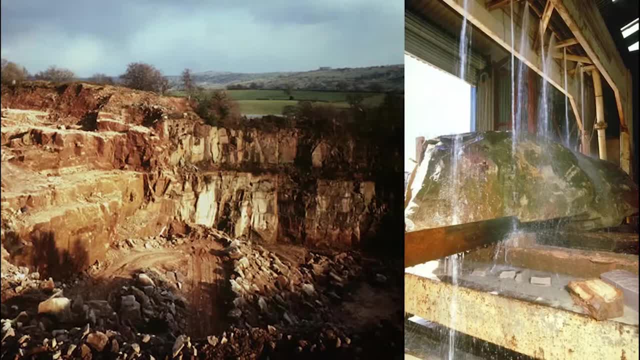 else. so for the stone columns they wanted to use natural stone columns. so here this was an opportunity to learn from first principles about how a natural sandstone material works. there is no code really for this. there's some guidance in some of the masonry codes. there's some guidance from uh places like the institution of structural 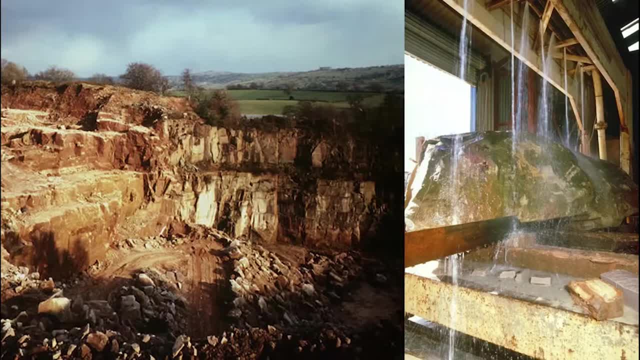 engineers, where there's, there's academic papers, but really we were trying to use a natural stone in a, you know, in a modern environment and make it safe and robust. so we went through a process of understanding, of testing the material to understand how it works. really we needed to. 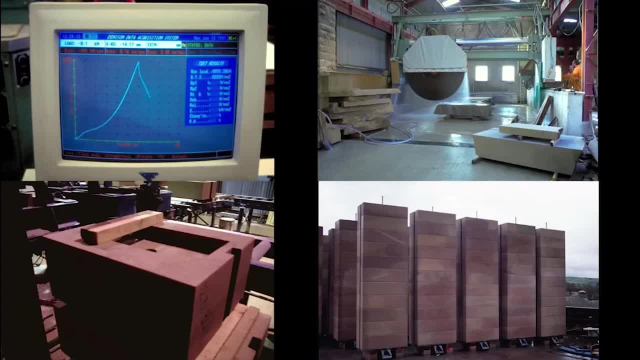 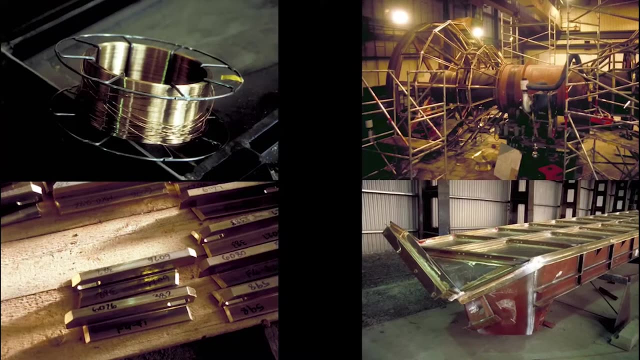 understand how it was made. so we spent a lot of time with industry, really using their knowledge to inform our design, and then together we created something that was quite unique and quite special. another component of what we did on the portcullis house was the bronze roof aluminium. 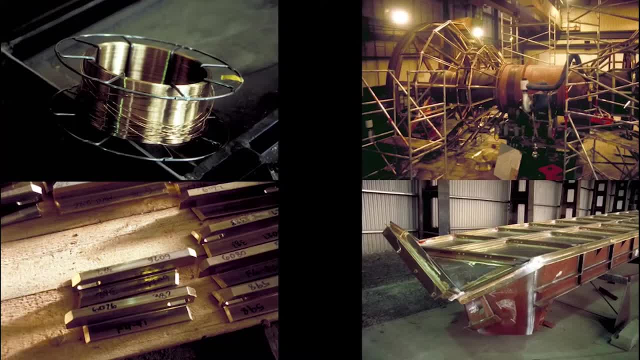 bronze roof with a bronze alloy. and here we chose to use bronze because a lot of the roofs in and around westminster have bronze finishes, but there was other reasons for it. in terms of that, bronze is a very durable material and, in terms of the roof, would require little to no maintenance. 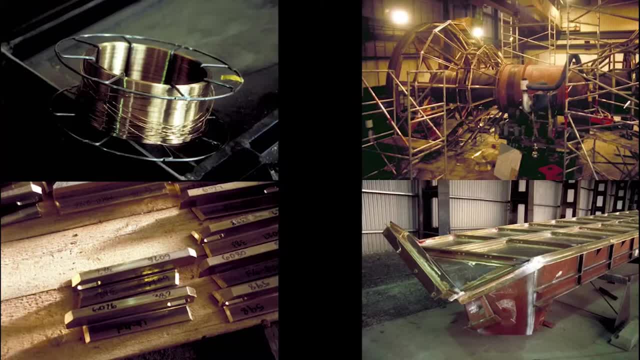 but what was interesting for me about this particular material was that it had never really been used in the construction industry before, but it had been used in other industries like the shipbuilding industry and the offshore industry. so what i thought was really interesting about that was the opportunity to 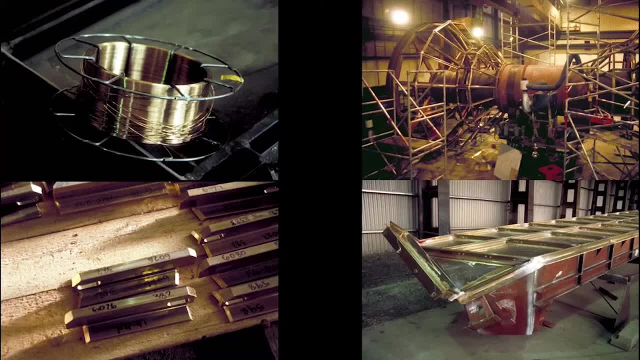 transfer technology from one industry to another. i think that's an opportunity for us going forward. it's about how we use technology transfer across a whole range of industries to inform what we do today and do things better. and again, for this particular thing, there was no codes of practice. 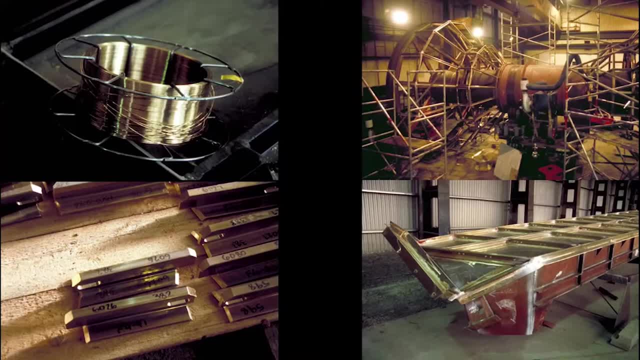 there was no standard specifications, there was no standard details, there was no standard welding procedures, there was no standard bolted connections. so, basically, we had a blank sheet of paper and a new material and we created a design, specification and drawings that could be built on site in the city of 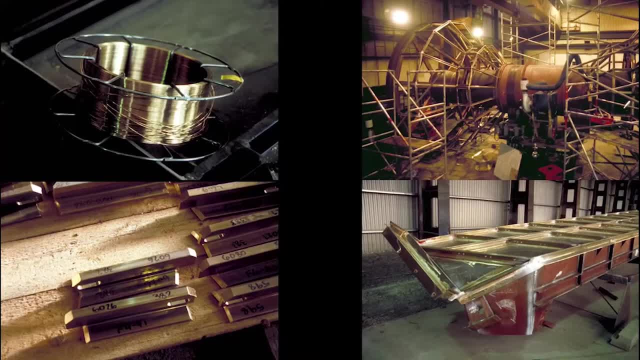 westminster, and that's what we did. so it was an opportunity to really get down to the that, really literally the nuts and bolts of it, and understand how things are done. a fantastic learning experience that i've used right throughout my career as i explore materials from a first principle to a. 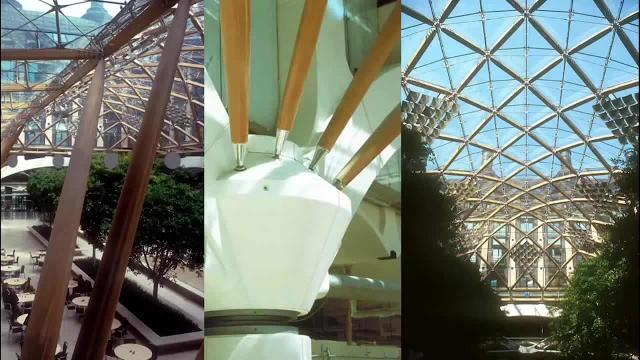 new approach. now you might say, well, this isn't a new material, it's timber, a beautiful material. but what we were trying to do here- this is the courtyard of portcullis house- was to replicate, i suppose, a bit of homage to the great hall in the palace of westminster itself. so it's an 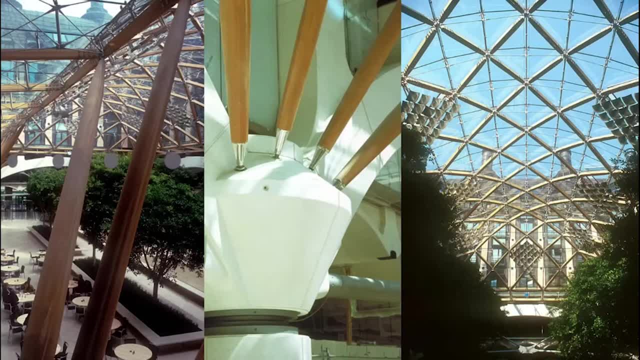 interesting juxtaposition of the old and the new. so we're trying to do a modern interpretation of the timber roof in in the palace of westminster, and here the architects wanted to use an american hardwood, which was a design guide that we developed with the american hardwood council, which is a design guide that we 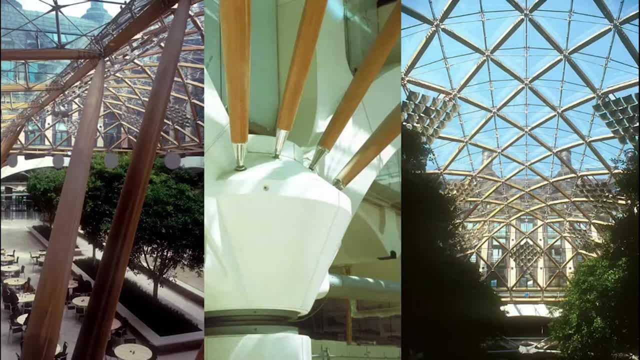 are trying to achieve. but again, there was no data about the uh, the allowable stresses that we could use um for for american hardwood. so we, actually we- collaborated with the american hardwood council to embark on a series of testing and research to understand how that material performs now as a 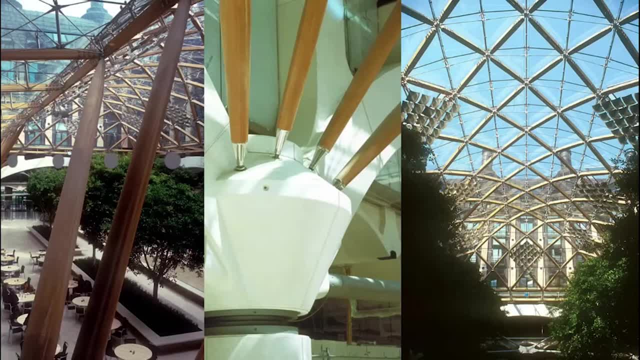 result of that, we achieved the design, but we also developed, with the american hardwood council, a design guide so that information was available to others. so it was about giving back to industry as much as learning for ourselves. i think that is something that is important and if we're trying to 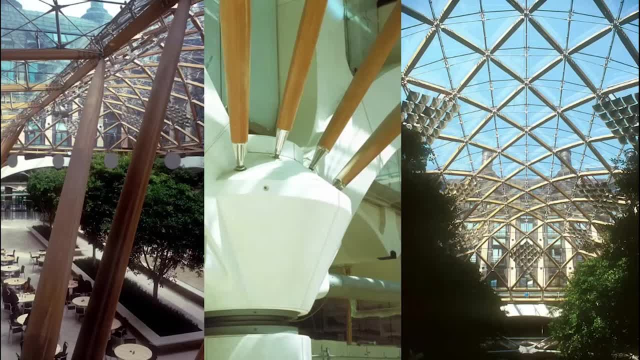 address some of the challenges that martin was putting to us earlier on. i think this idea of collaboration and the spirit of sharing knowledge and helping each other um solve the the the the problems of today, i think is hugely important and in the end we got what i think is a wonderful 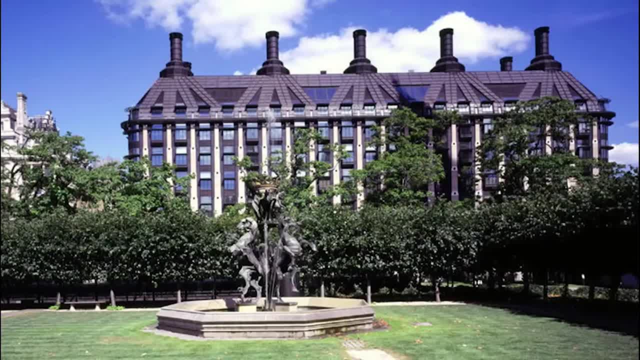 project and see if we can get the i don't know where, the which one is, the uh, these pointer, oops. so the bronze roof. on the top you can see the natural stone columns in the vertical structure. they're, uh, post-tensioned. and then you can see the nodes of the, the concrete. 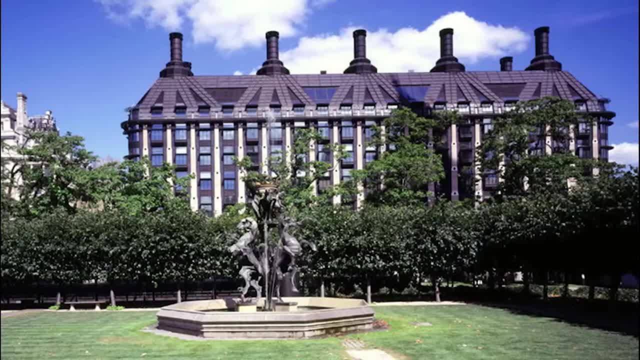 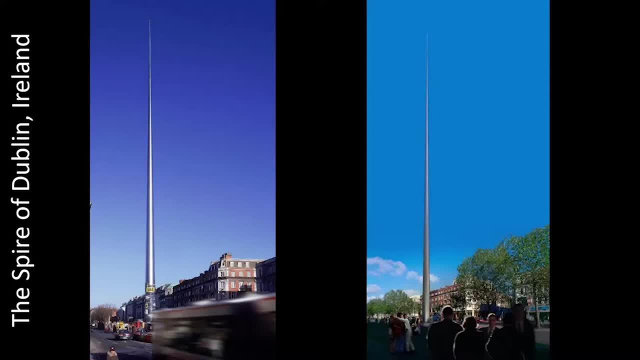 elements coming out. so that was my first, i suppose, big experience of thinking a little bit differently and beyond code, and that quickly led on to this project, which is the spire of dublin, which is basically: it is a sculpture, it is a piece of art, and that that's the way it was presented. so when 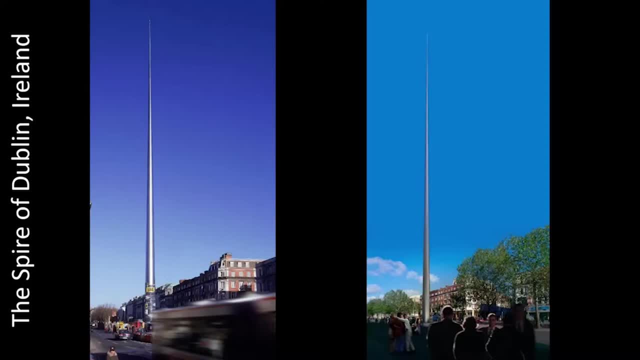 you were speaking to the architect and the client about a piece of art. the language changes quite considerably, so it was all about the thing, finishes, the tolerances and the finesse of what you touch and feel and see. but also it's a big piece of complex engineering. i know it looks simple: a cancer lever, you say. i'll have one. 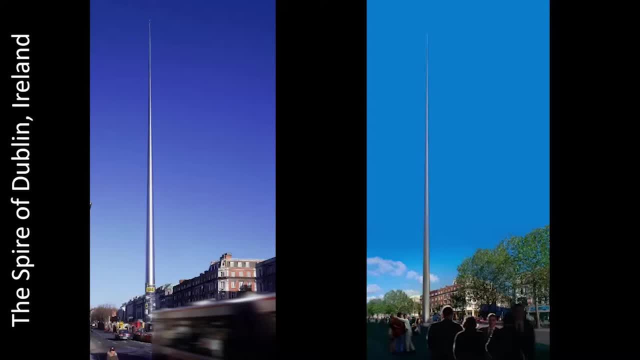 of those every day of the week in the structures exam. it's easy. but it's 120 meters tall and it's three meters diameter at the bottom, so it's very, very slender and it's 125 tons overall. but the issues that we had to resolve from an engineering point of view was win dynamics, fatigue damping. 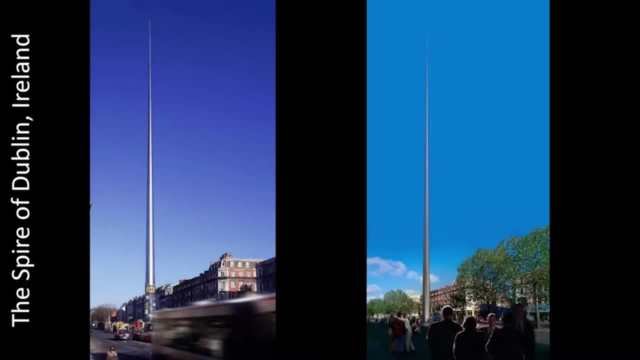 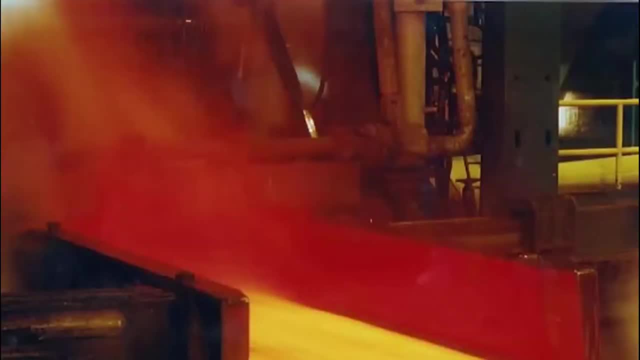 the whole lot, not something that came up in the discussion with the architect or the client. they didn't see this as as an issue. they just saw the art pieces, what they wanted to achieve. but actually to achieve the engineering, we needed to understand the physics of the material, how. 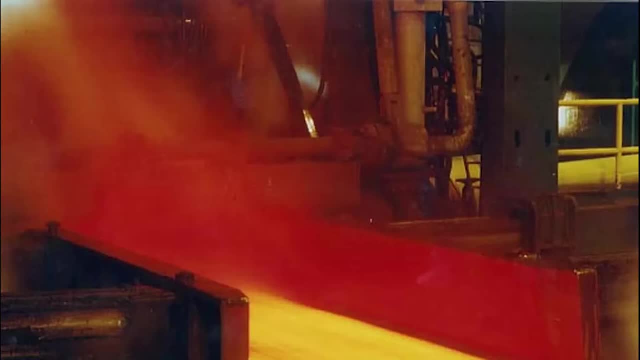 stainless steel, how you know what's the natural dumping of it, how does it behave in a fatigue situation? how does it behave in wind? but then to achieve the aesthetic of the piece, we really needed to understand the essence of the material itself: how it was made, how it was worked, how it 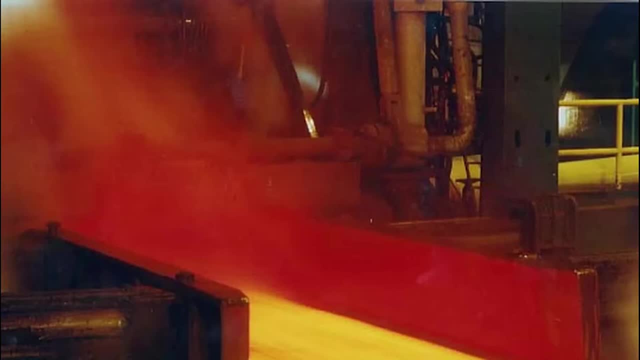 was prepared, how it was fabricated, how it was put together. there was some guidance out there, but not a lot. but again, we use technology transfer because stainless steel is used a lot in the pharmaceutical and the food industry for high levels of polish and finish. so we got a lot of information from 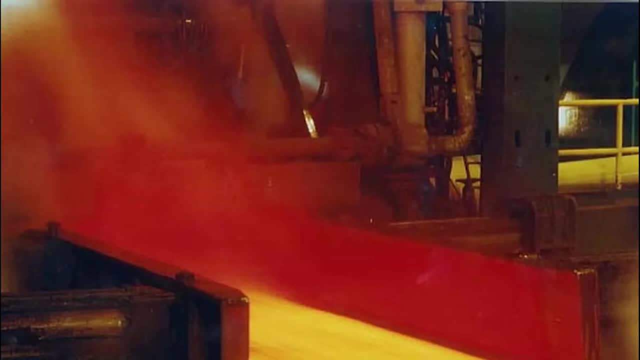 that industry to inform the finishes, and i'll go through that a little bit more. and we also had some technology transfer from the f1 industry. so that's quite interesting, the f1 industry informing the building construction industry, which is quite special. so we got back to really in first principles understanding from 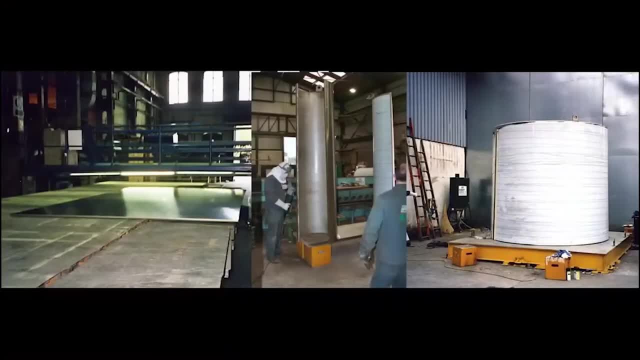 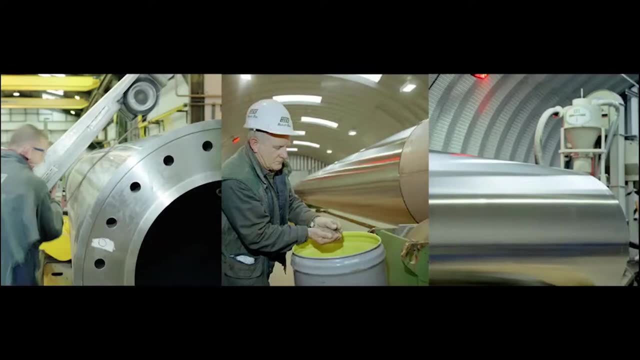 when how the material is rolled, how it is flattened and made, how it is curved, how it is polished and finished, and then um this piece. here is where we got the technology transfer from the f1 industry. we shot, peened um the the, the spire as part of the finishes, but actually the shot painting, work, work. 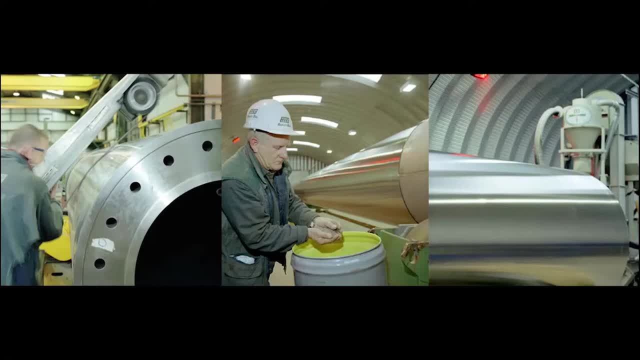 hard in the material as well. so it actually helped us in terms of the fatigue design that we were trying to undergo and that there was papers from the f1 industry that allowed us to make an informed decision about that particular approach, and the thing that came out of it at the end was- um, you know, it got a lot. 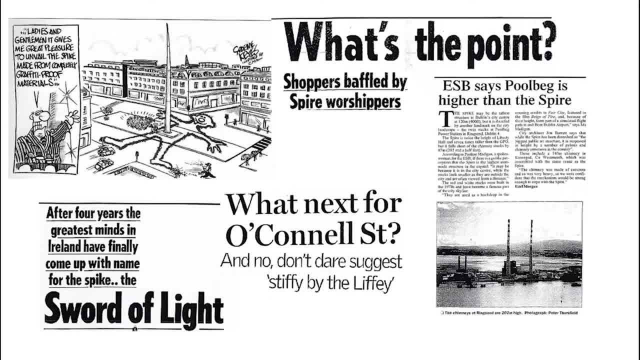 of got a lot of press for all the right and wrong reasons. um, it got a lot of debates amongst the people of dublin and ireland and dublin, which was at its best when they started coming up with various nicknames for the spire, but also at the end they created a project that was quite beautiful. 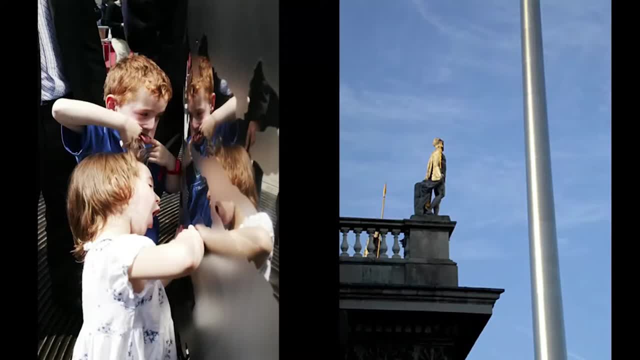 it was part of a city generation project. it kind of um endeared a lot of civic pride. the people of dublin might give it a nickname, but that means it's got a place in their heart, so it really garnered some civic pride. it created joy and 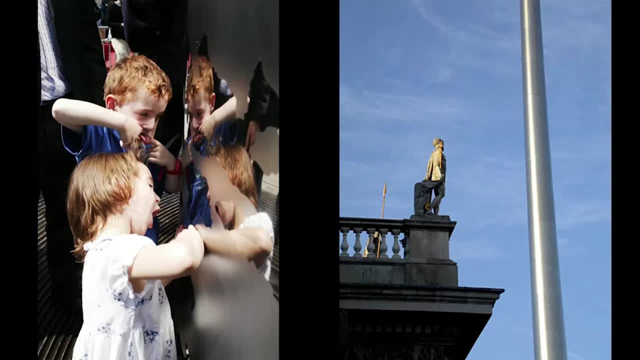 delight. the feedback we got from the, from the people of dublin, was fantastic. you know people coming up to say thank you for creating this wonderful piece. so there was a piece earlier on about how. i think one of the discussion points is how do we give profile to engineers for things. 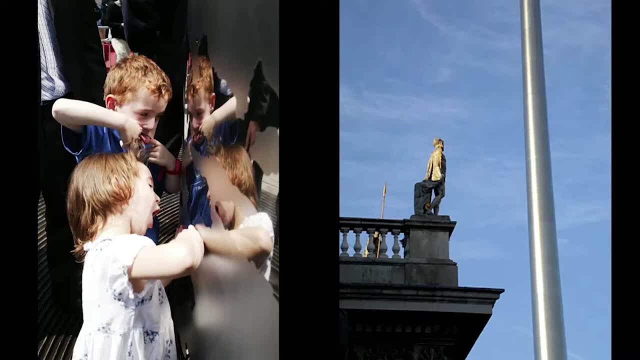 other than a disaster. things like this, when we do it properly, um give us that opportunity to to to, to raise our profile, but also the knowledge sharing. some of the research that we did to deliver this project has been. it was published in the ice director structure engineers journal. 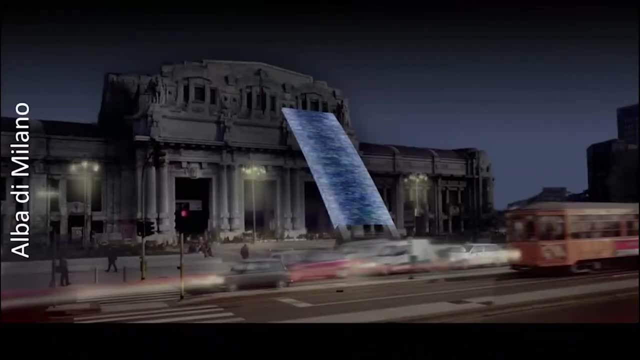 has been used on projects around the world since. so they were the two of the big sort of projects that i was really got my interest going about materials, and then that quickly moved to a whole pile of projects and this is one that we did in milan and the material here. that was quite of. 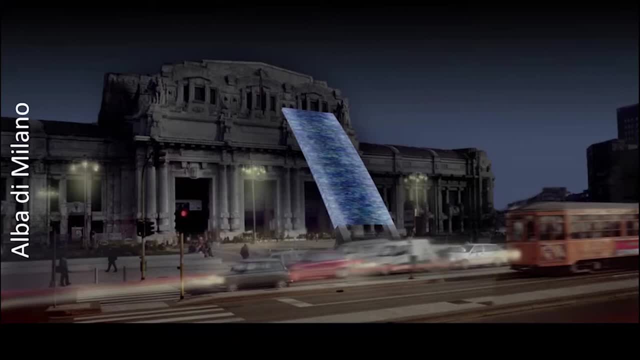 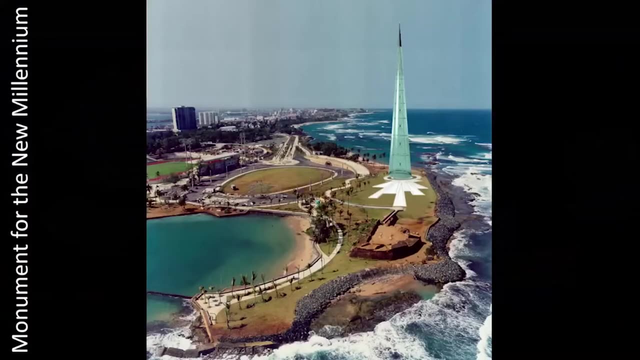 interest was a woven fabric that we created through fiber optics and stainless steel wire to create this kind of light canvas that could be part of a piece of art and sculpture. this is one that i did with the, the architect that came second in the spire of dublin competition. 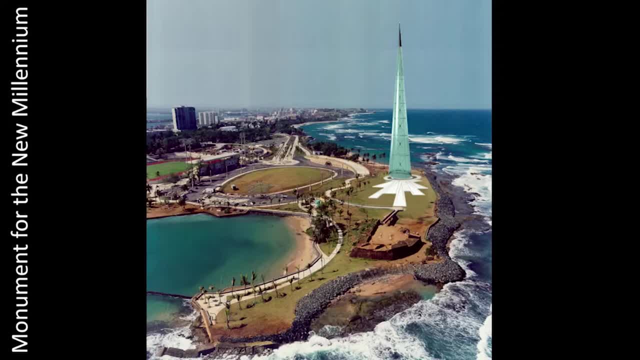 this came up a little bit after and he said: okay, you won it the last time, maybe if i team with you i might be first this time. and we didn't win it, but this was a 100 meter tall recycled glass tower in a seismic area, so maybe coming first was a blessing in disguise for us. 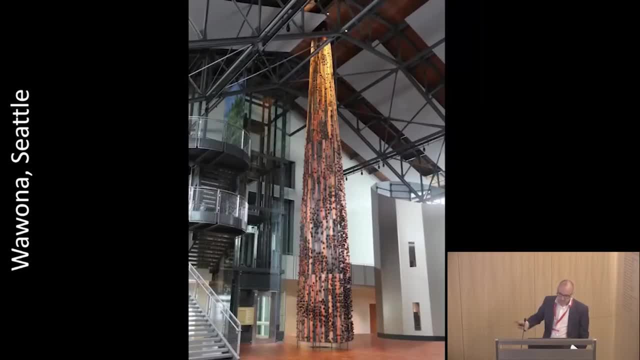 very, very complex piece of work. and then this is more recent. it's a piece of sculpture in in seattle called wawona. it is a piece of art. what was interesting here is about upcycling. so all the materials from this was from a schooner that was rotting in uh in south lake union, in in washington. 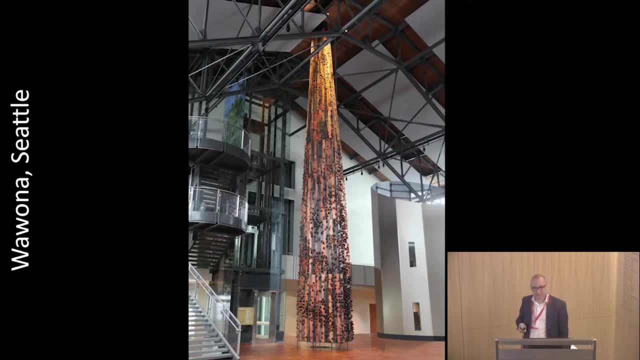 and the museum- the local museum was- was part of their exhibit. they were going to get rid of it. and an artist said, no, i've got an idea, and it was an idea to kind of recreate, kind of be an image of the hull of the schooner um in as a piece of art, and he worked with us to do that but to achieve it. 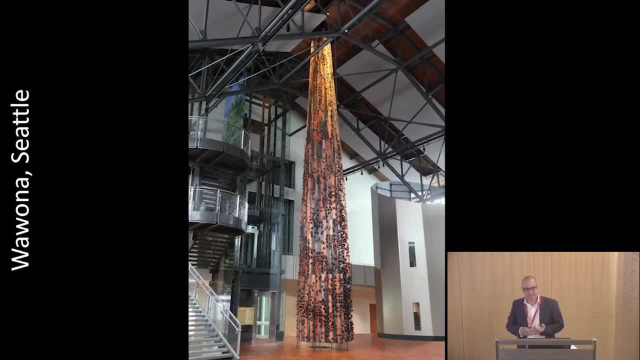 had to understand the material that was about 300 years old, how it had decayed after so many years rotting away in the water, what the material strengths were like. so we worked with a lot of academic researchers to to understand that and then when we got into kind of creating the piece, 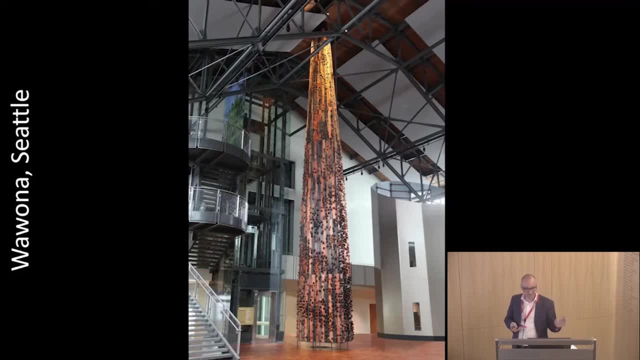 itself. we, it was really design and fabrication, digital design to fabrication process where we designed with the artist all the features on the outside and that went straight to a five-axis cnc created. so it was direct from our analysis and design software straight into the software of the. 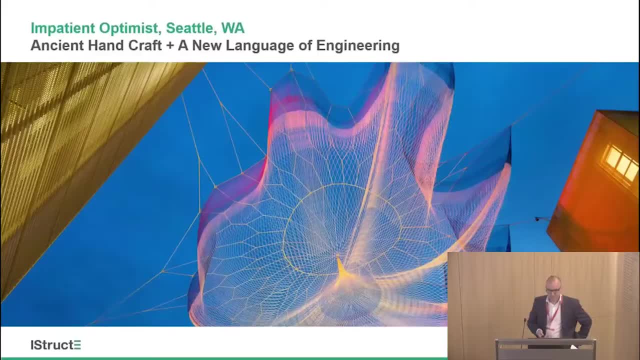 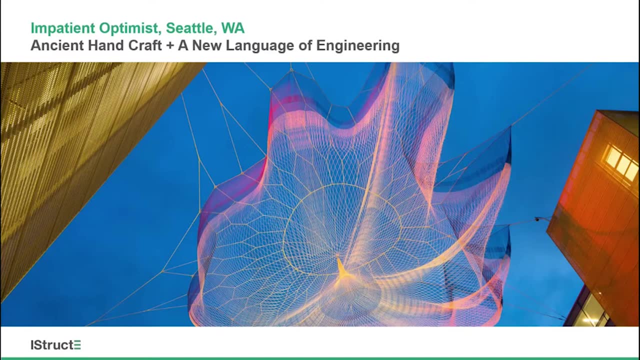 of the fabricator and a beautiful piece. so that's a little bit about my journey and, uh, it came, i suppose, culminated, a couple of years ago and this is one of the projects i think that elizabeth was talking about at the start, and this is a project called impatient, optimist and 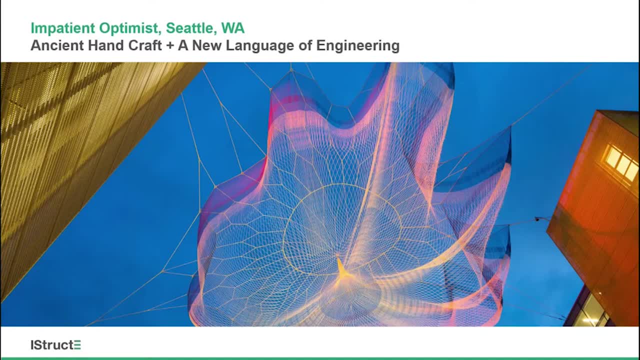 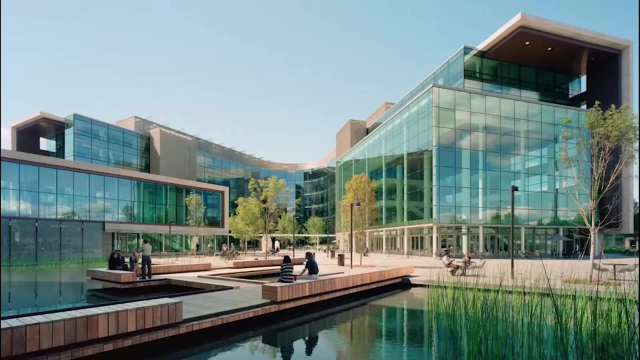 what i'm going to talk about here is about how we mirrored an ancient handcraft with a new language, and i'll take you through that right now. so we had just completed this project in seattle, and it's the new headquarter building for the bill and melinda gates foundation. it's a campus. it's a. 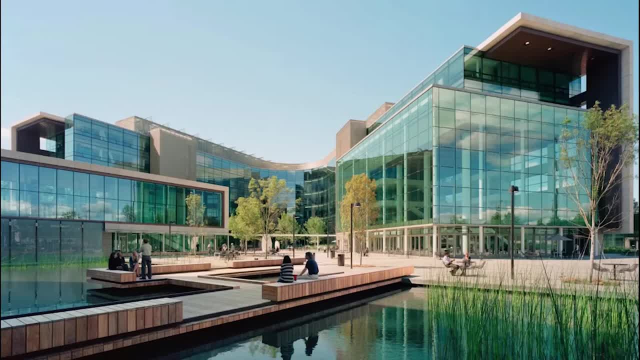 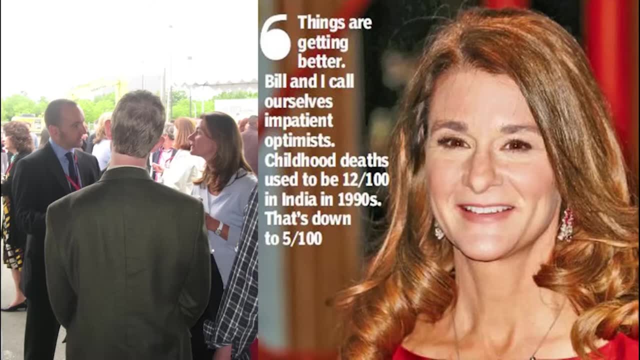 city center campus consisting of three projects and a wonderful plaza in the middle, and this is melinda on the right, and they- herself and bill- call each other the impatient optimists. they're very optimistic about the change that can be made to better the lives of many people around the world. 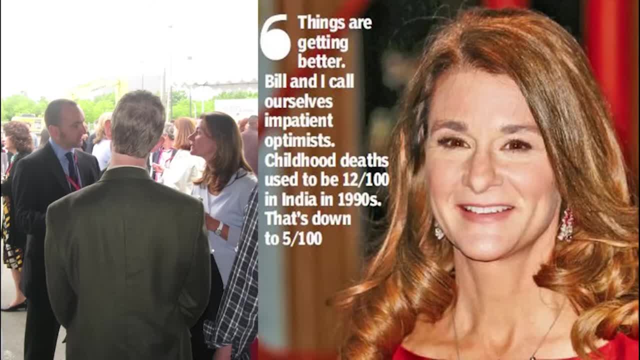 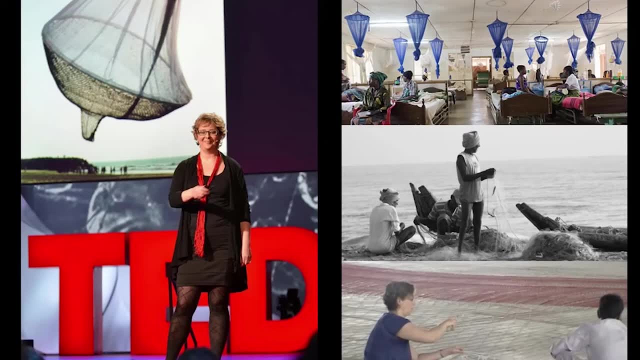 and they just feel they cannot do it quickly enough. but melinda was very interested in the art of this woman called janet eccleman, from boston, and janet was a fulbright scholar who went to india to study art and she was really intrigued by the fishing nets of the local. 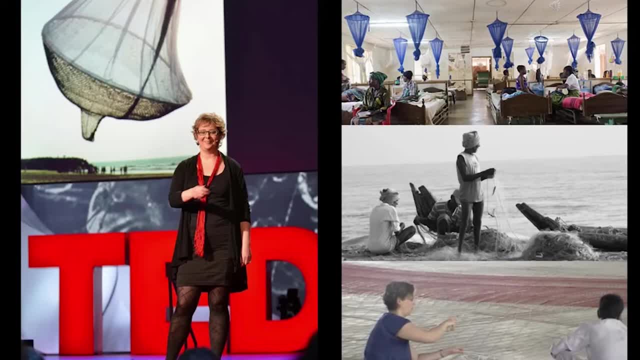 fishermen and when they finished the day's work fishing on the seas, they used to come out and dry and repair their nets. and what she really likes is this kind of space that those things created. they created kind of a transparent space where the workers would talk, eat, fix their nets, but it was their own little environment, but it was open for everybody. 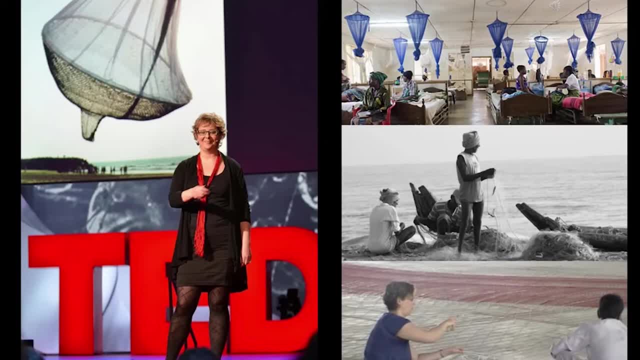 else to see what was going on. she also liked the way that it blew in the wind, and this was. this is part of her artwork. she's been doing this kind of theme of stuff for many, many years. melinda wanted one, i liked it and wanted one for the campus. so basically, the commission. 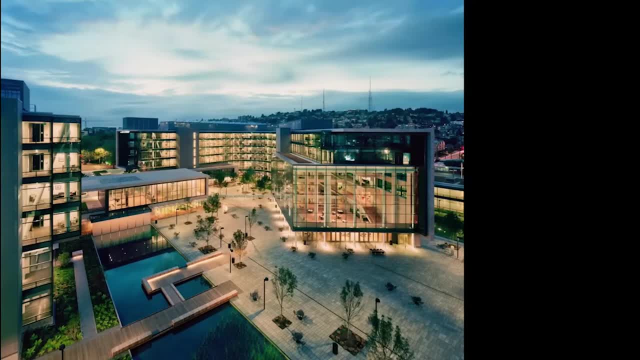 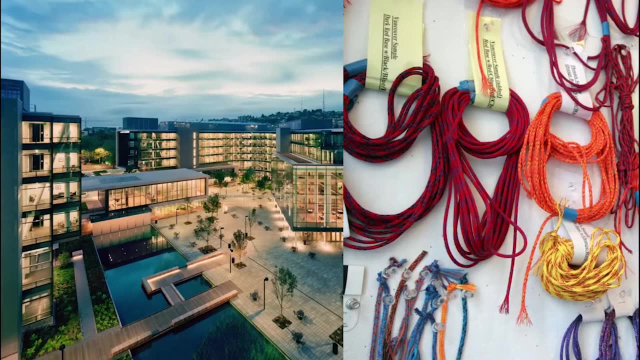 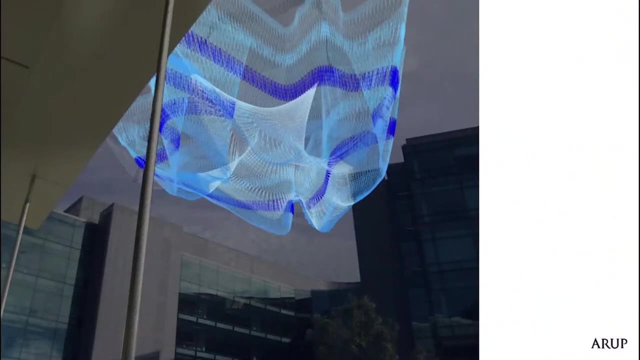 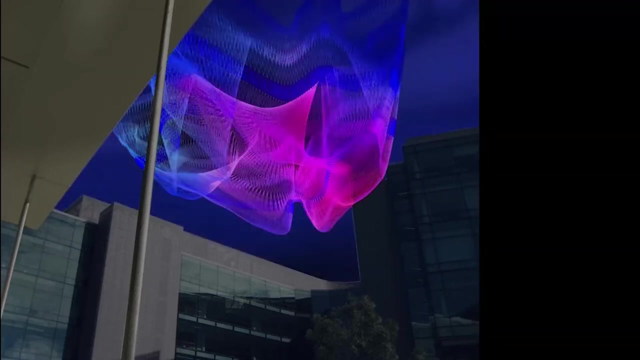 was to create this piece of sculpture hanging over the public plaza in this campus that we we spent many, many years working on using a palace of materials that looked like this rope and wire. and then, just to add to that, the, the illusion I was sold to the to Melinda by Janice, was this beautiful net that 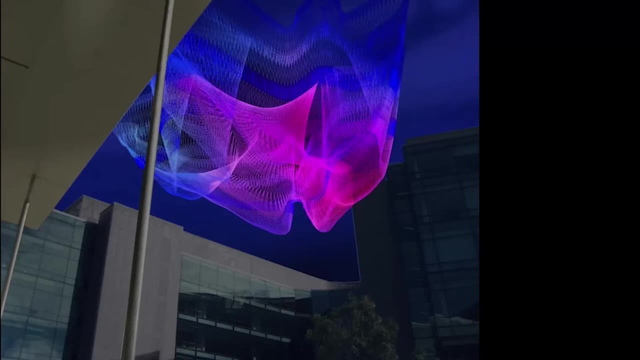 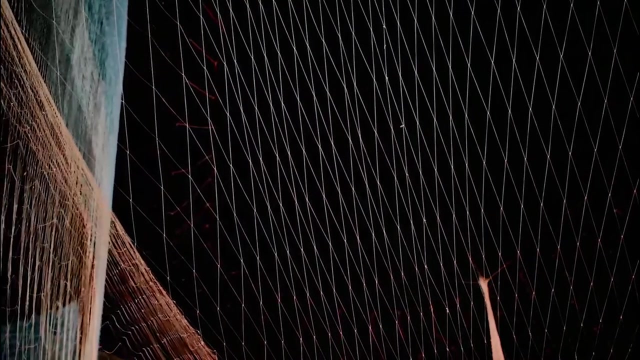 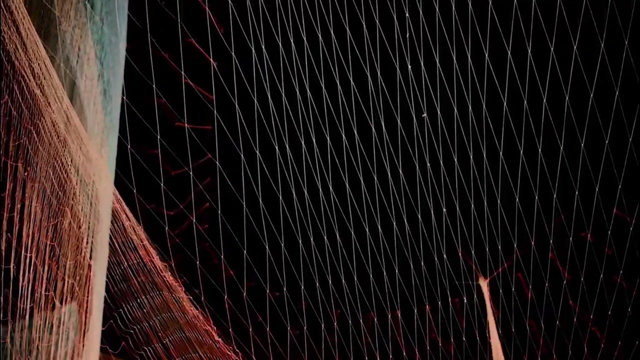 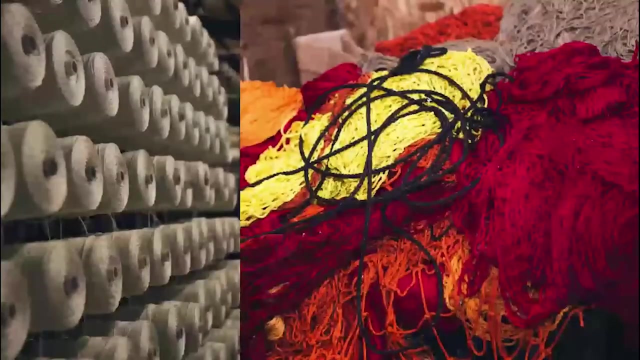 floated in the breeze and changed color with different lighting. and then there was this little video. if I can get it to work, let's see does that work? so this is the effect of it: kind of blowing quite gently. so wonderful vision, developed through computer software, sold to a very influential woman, Melinda Gates, and just 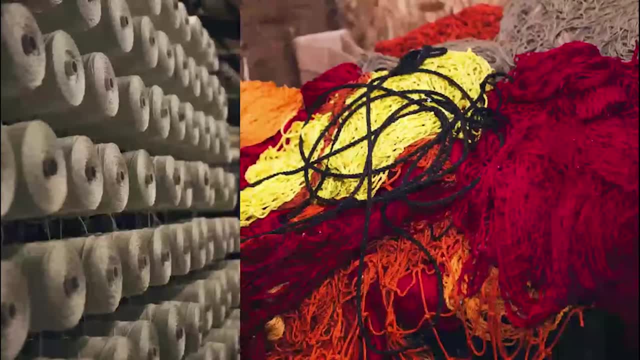 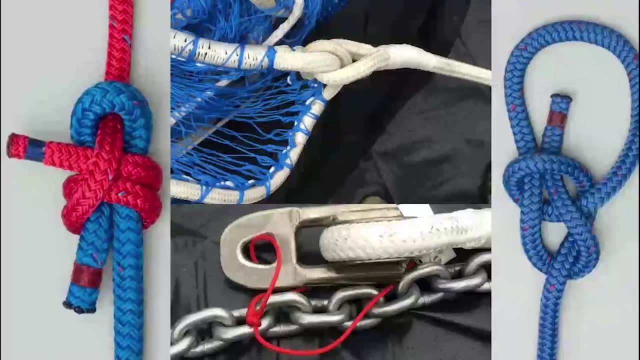 to remind you, this was the palace of materials that we had at our disposal, and then we had a couple of stuff that we could test a little bit more. you know, there was from the sailing industry to bind some of the ropes together and connect them. but this is. 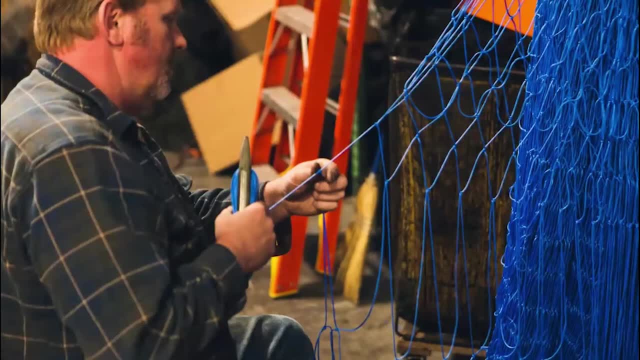 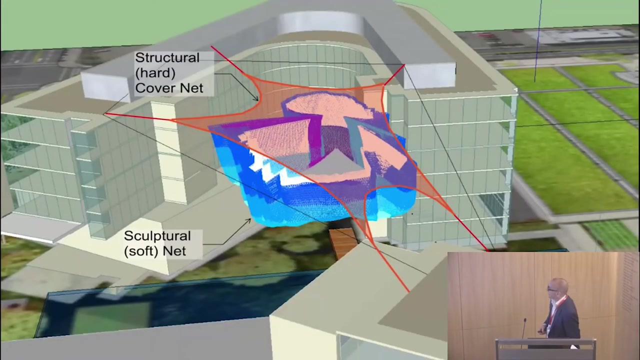 how it's made. I mean, these are the guys that made this. their main business is making fishing nets. that's what they do, but it was that ancient handcraft of making fishing nets is actually what's instrumental in Janice Akelman achieving her pieces of art. it's very, very basic. so this is what we had. we. 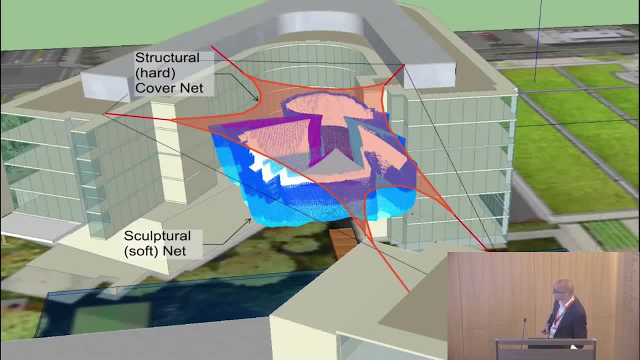 broke the structure at the sculpture down into two main components. we had what we called the favorite giant sailor, we call it the ultra double sailor, or the called the hard net or the structural net, which is the piece spanning between the buildings, and then we had the sculptural softness which was hanging. 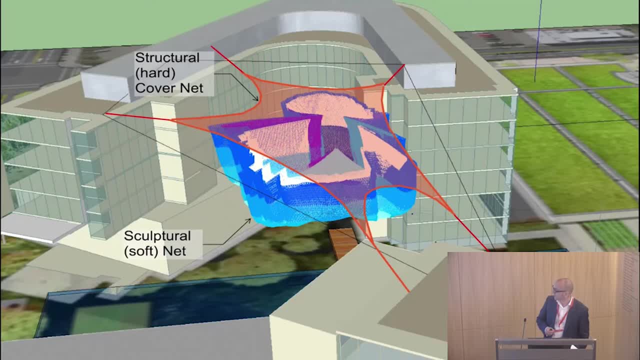 beneath it and flowing and hanging over the public plaza. the geometry is quite complex, the materials are quite complex. the dominant loads on this is wind and snow and ice. so we thought: how do we approach this, bearing in mind how it was made? how do you approach the design? and then, once we design it, how do we pass on? 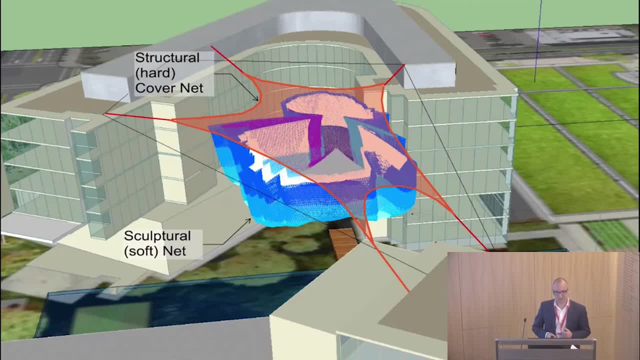 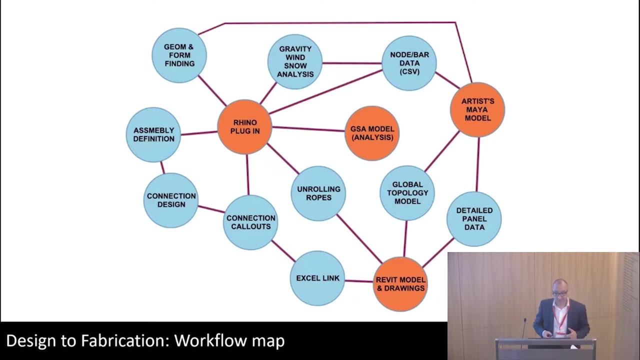 that information to the people in the workshop to make it so it's really coming together: complex analysis, communication of design and implementation of the outcome. so, jumping ahead a little bit, this is what we did. we kind of digitized the hell out of it really. we kind of automated as much. 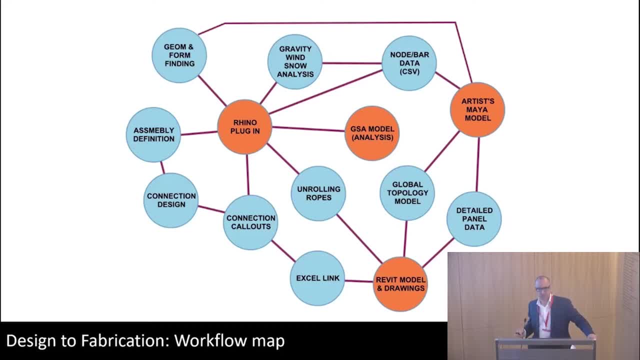 stuff as we could, and the reason we automated- not just because we could, because it's actually what made sense, it was the right thing to do, you. but by automating a lot of the complexity and a lot of the really iterative sort of stuff, it gave us time to think how we would actually prepare. 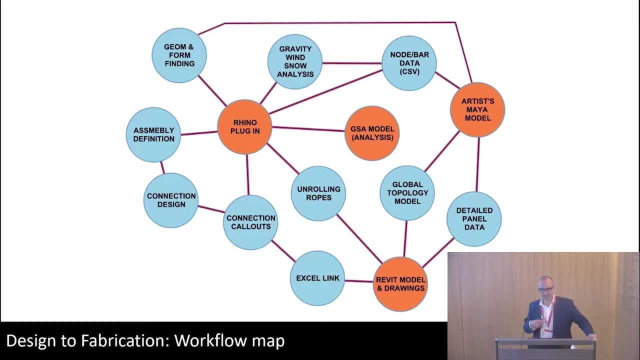 the materials for the people to make it. it would allow us to focus on the things that added real value to the overall piece. so the pieces in orange are the kind of the main sort of tools that we use to drive the input and the output, and the blue is what we got as a result of all that. so a complex workflow map. 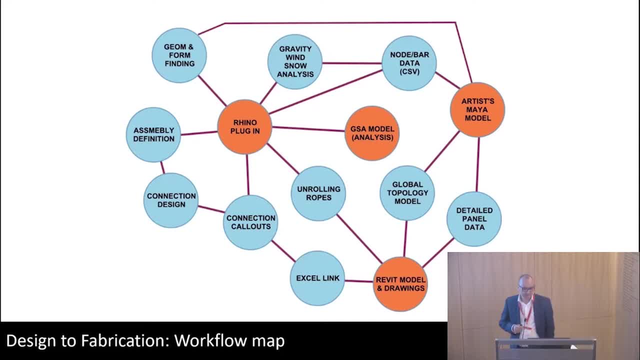 that was created by brilliant engineers and we were able to get a really good engineer for my team in Seattle called Clayton Binkley- absolutely amazing guy. but the whole idea was really to try and take this digital environment, get it to fabrication in a way that could be understood by the workmen. so, as part of 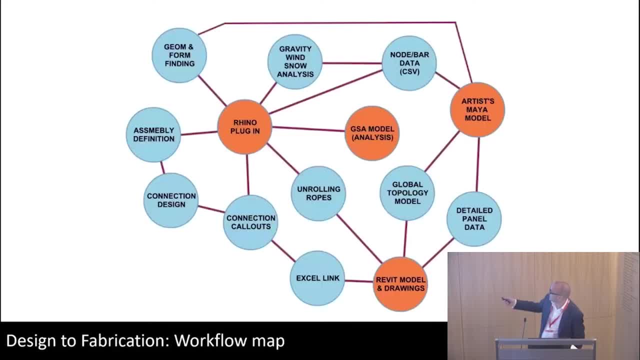 one of the big things that a lot of the software was already there. there is the Maya toolkit for Janice Ackleman to put her stuff in there. Revit obviously was available and GSA is the structural software that Arab uses. it's in-house software that we use. that is. 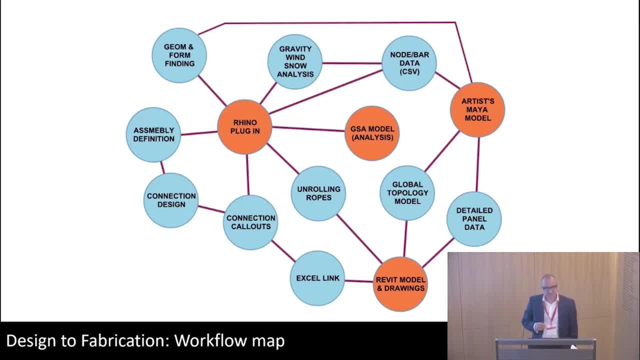 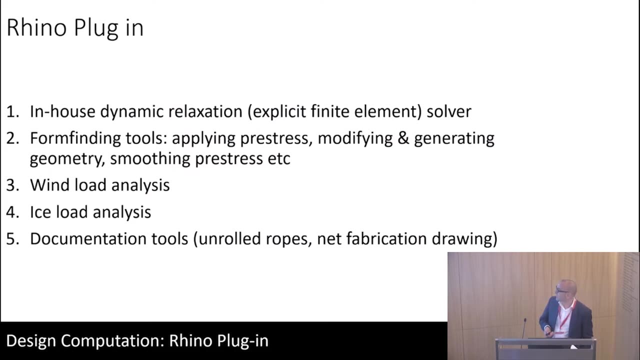 available if you want to buy it. but the Rhino plugin has actually well connected the whole lot together and actually allowed us to do things like the wind loads, pre-stress, form-finding and everything else. so this is what the Rhino plugin did. it was a dynamic, in-house, scripted, dynamic relaxation. 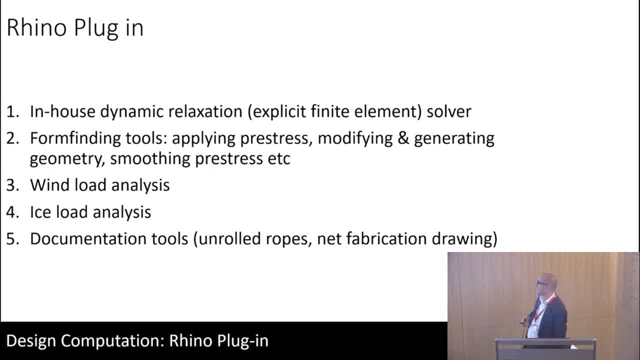 solver. it allowed us to do the form-finding for the, for the net, applying pre-stress and modifying and generating the geometry as a result of the pre-stress, then smoothing out the pre-stress. and this was an iterative process because every time the geometry changed we had to, you know, go full. 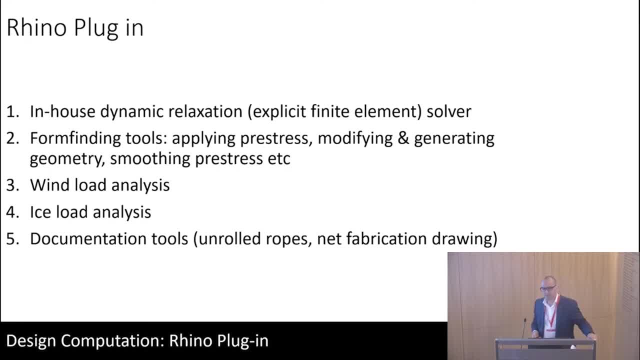 circle with with the artists to make sure it was in line with it what they wanted to do. once we had that, then we were looking at all the the wind loads, that, the ice load analysis and then finally the documentation. so this is really a complex 3d piece of structure and we created tools within the Rhino. 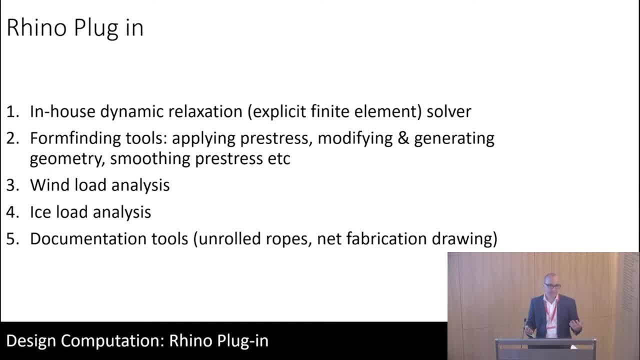 script to unroll every single piece of it. so it became a 2d image like a pattern that you'd make closer thing out of. and that was our aim and that was the way we felt we could document and communicate the design to to the workers. so this is kind of the 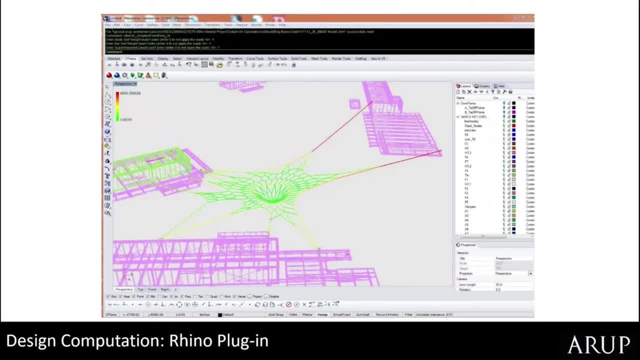 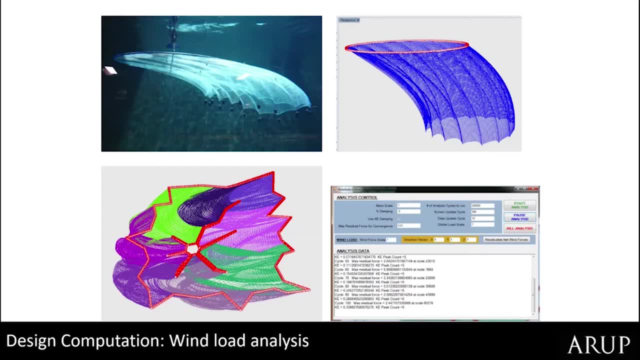 script and the plug-in in action, not going to go through it, but the this is a little bit and I'm just going to touch on this a little bit more- where you know, we try and understand the physics of the material and the physics of behavior in 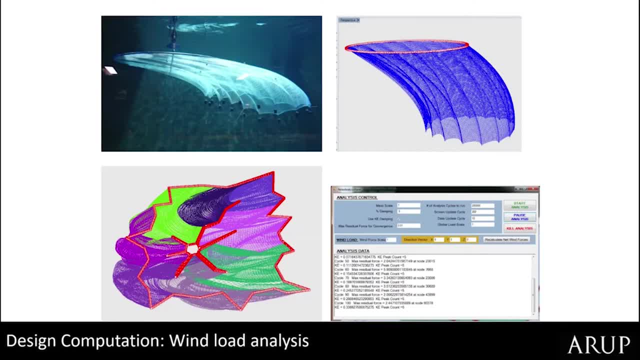 external environments and that, in wind, behaves quite differently down the say, a building. so there's very little stuff out there as to how we would approach it. so we spent a lot of time looking at the impact of wind on the knots, the ropes, when it drifts and shields one part of the net shields. 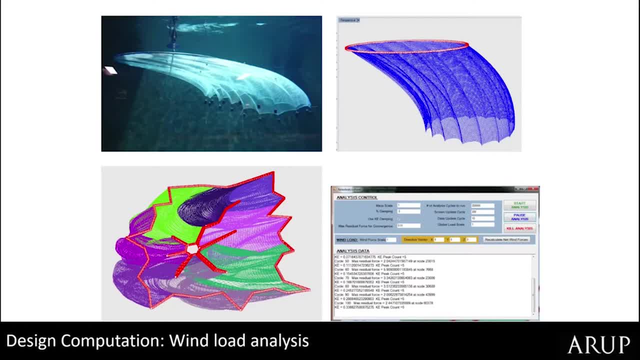 another part of the net. what's the change in loads? there's dynamic effects that we needed to come in into it, but there's thousands and thousands of elements that each behave differently, and that's what the script allowed us to do. the Rhino script allowed us to really iterate through that, really, really. 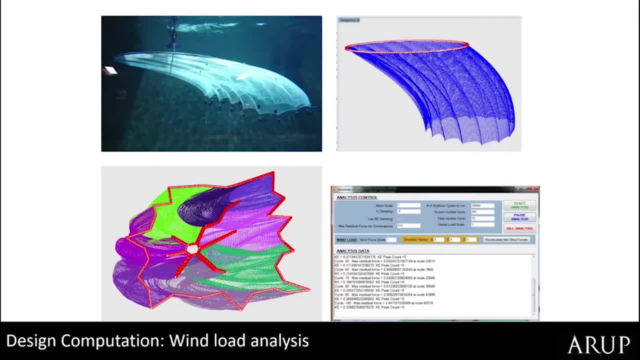 quickly. but what was interesting, the research that was done by the wind industry in Norway was to kind of progress it most in the most optimal way was research actually that was done in the fishing industry in Norway where they actually put fishing nets in tanks of saline water and put a. 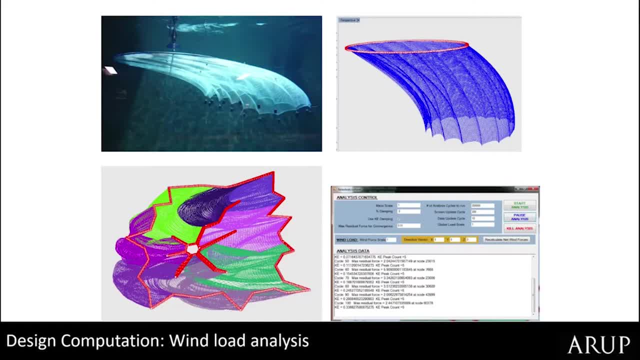 flow through them. so you could see how the fluid interaction with the net. it was the principles of that that we applied to reduce the wind loads that one might ordinarily expect if you take, you know, a straight interpretation of a current code. so actually, again, technology transfer from the fishing. 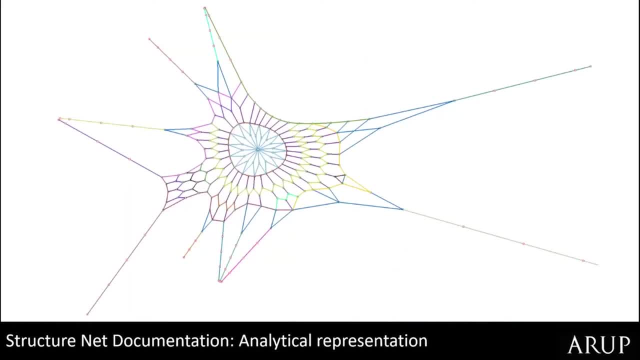 industry to the fishing industry is not about keeping the net in place for reference purposes, but it's about how we process that information and how we use it to retrieve something quite beautiful. so in the end we got this, and this is the, the analytical representation of the final model. but 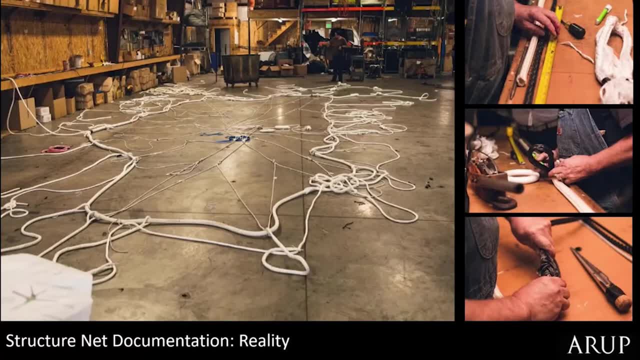 then how we portrayed that information back to the, to the workers, because this is how they make it there: they are pieces of rope on the floor, they get a tape and they measure it and then they cut it and splice it, and that's what they do. they don't use spreadsheets. it definitely don't use Rhino, so we had. it was really important how we 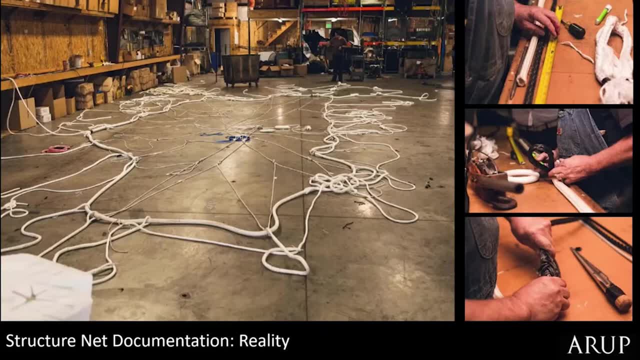 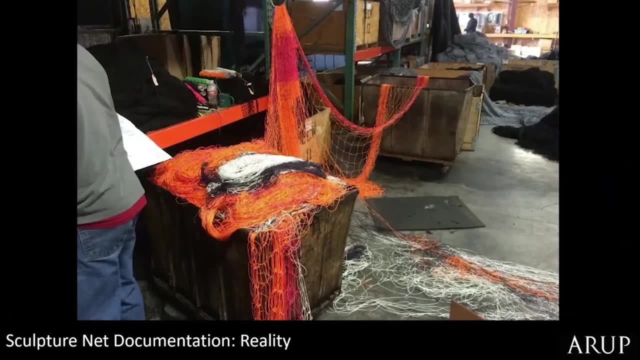 portrayed that information. also, we had to get in things like tolerances, connections and everything else, and then, as I said at the start, there was the pieces about difference of color. this is one of the nets being made with different, different color palettes through the net. how, again, do we portray? 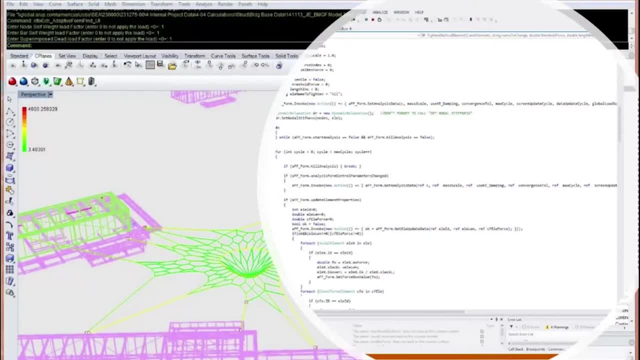 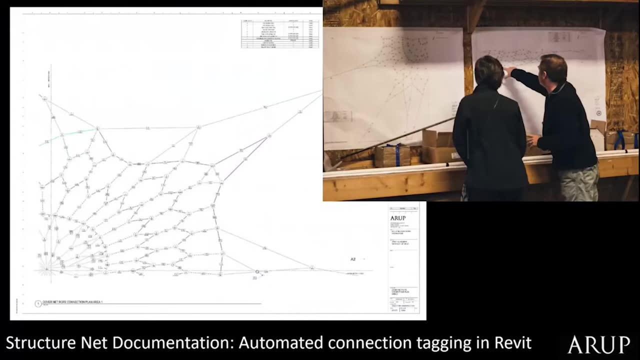 that information and this was not going to be the approach. we ideally want to give him the Rhino file, but that wasn't going to work. so what we did was we, as I said, the plug-in, unfurled all the nets and created a 2d pattern, and this is one. 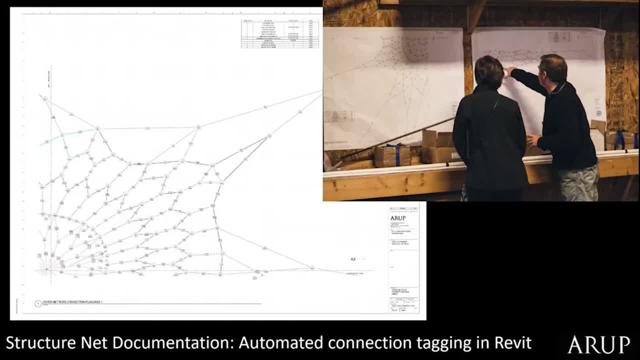 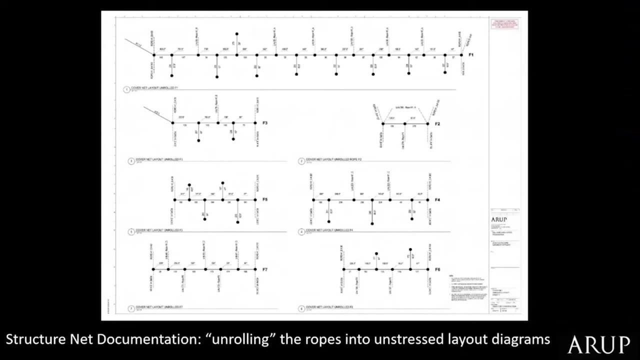 of the drawings on the left-hand side that we created, that basically unfurled a piece of net and all on that I did the automatically generated the type of rope, the length of the rope call out for the connection and they put it on the wall, as you see on the right-hand side, and that's how they made it. and then to go. 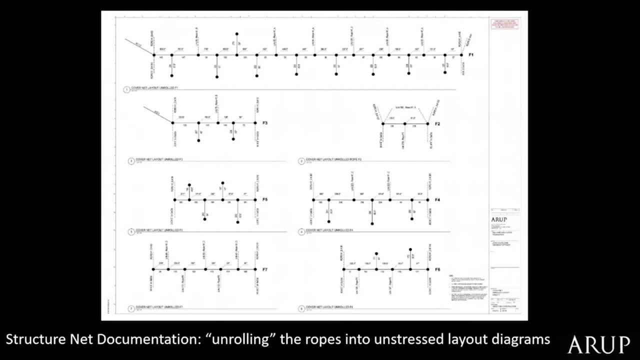 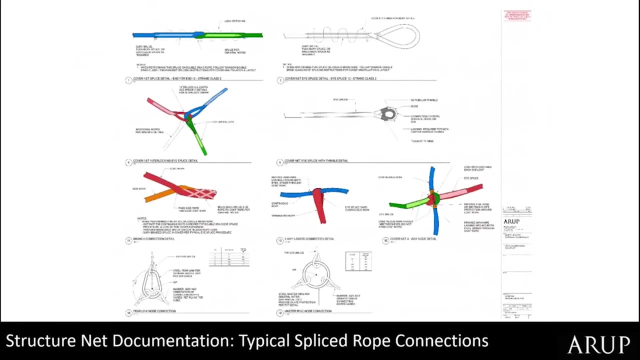 on to a little bit of further detail for the for the longer structural ropes we again called out where the connections of this softnet hanging and they could measure them out as it just a linear dimension on the on the group on the floor. and that's that some of the details we did for the for. 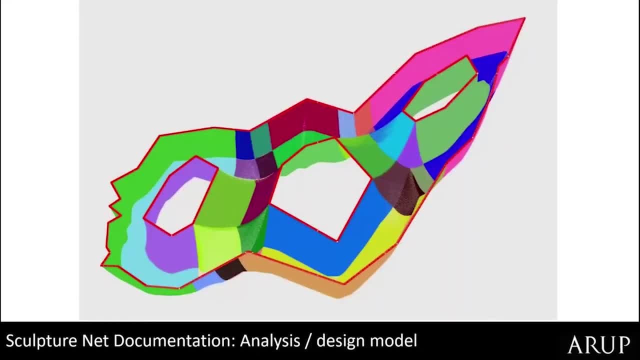 the connections. so to add to that, this is one of the pieces of output from Janet's software, the Maya plug-in that was developed by older does for, and this is where she's beginning to look at the different colors of rope and twine that were used throughout the structure. so we had to again this overlay of new. 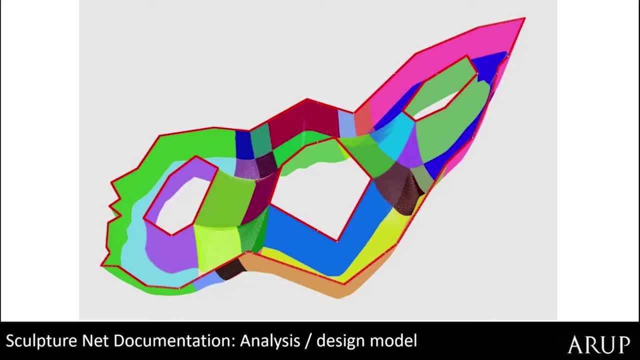 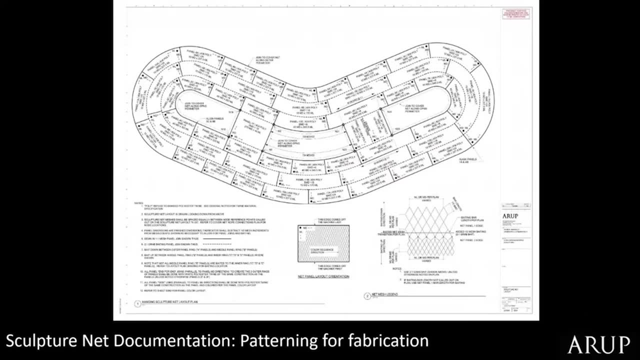 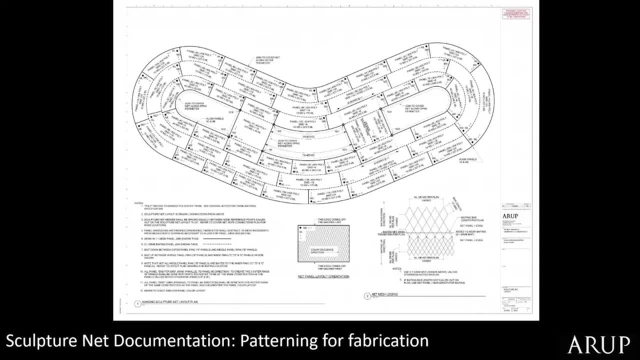 was about the adjacencies of the color palette. that's what was important in this particular drawing. but what is also kind of scary, I suppose, and intriguing, is that because this kind of creates the adjacent panels and how they have to connect them together in terms of color, because it's 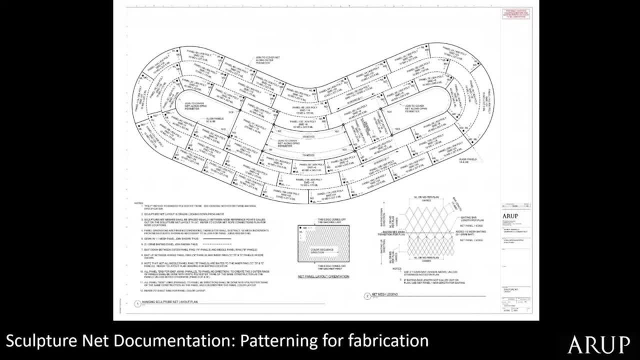 a 3d thing you never really see. there's no visual check that can happen along the way to make sure it's right. the first check you get that everything is in the right place it's when it's built. no shop drawings. you know nothing. you. 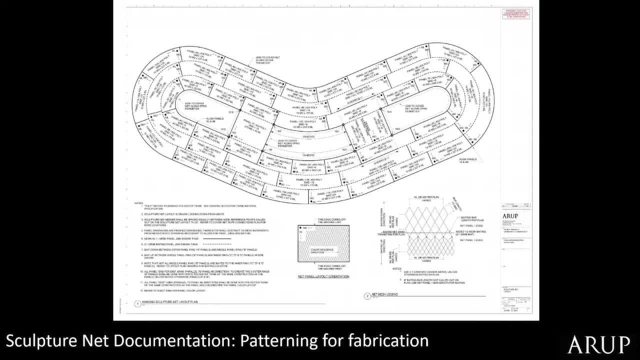 know you never see it in a 3d form to check it, so that is actually quite scary if you were to transfer that to a traditional sort of building. but it also talks about the relationship of trust. I think that's important when you stretch the boundaries of technology and what we can do so that the trust between the 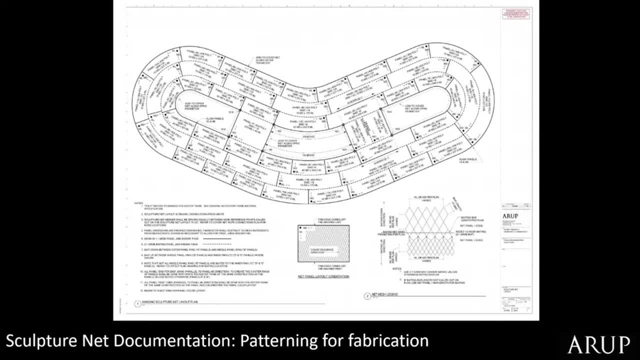 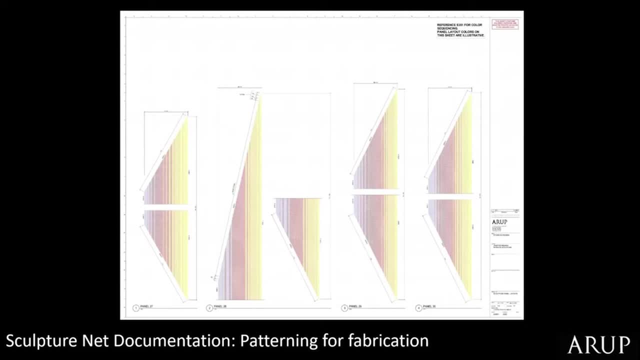 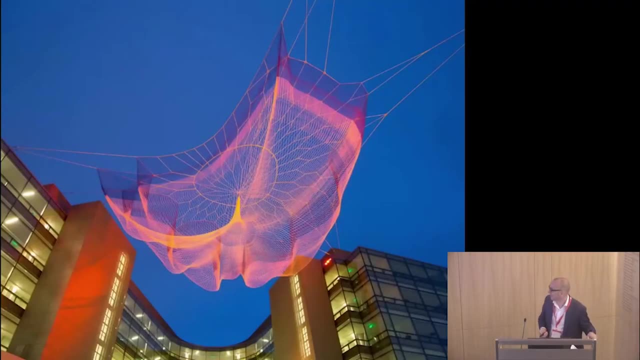 people making it, the artisans ourselves, was actually hugely essential to achieve what we did. so we again to help that, we kind of created the panels of different color and that came straight out of our piece, out of our Rhino model. but when you do it properly you do create a thing of beauty and this is the final piece. but 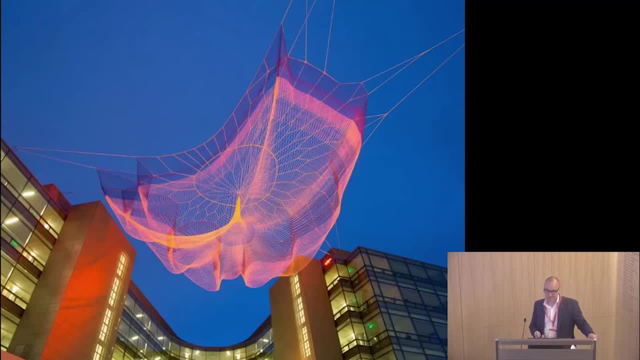 it was developed from all those like 2d drawings and information that we gave to to the, to the makers of the net, and then, when you get feedback like that from your clients, you think, okay, I've done something right and maybe inspired them along the way. 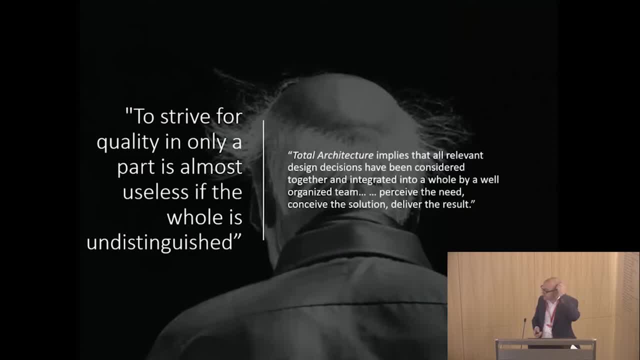 and this is a quote from, oh, from the key speech which I think is important and when I would talk about you know he says to strive for quality and only part is almost useless if the whole is undistinguished. when I think about our project, I think it is a beautiful thing, but actually when I think about quality, 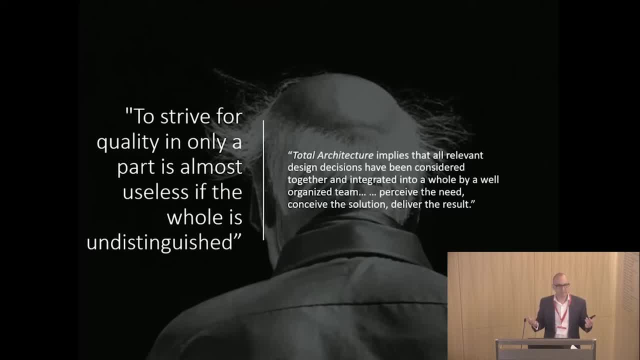 I think, if the quality comes out- and I think three main components, I think the quality of the relationship right across the client and design and construction team- that that quality of that relationship allowed us to achieve what we did. without that relationship I think we wouldn't have gotten where we wanted to. 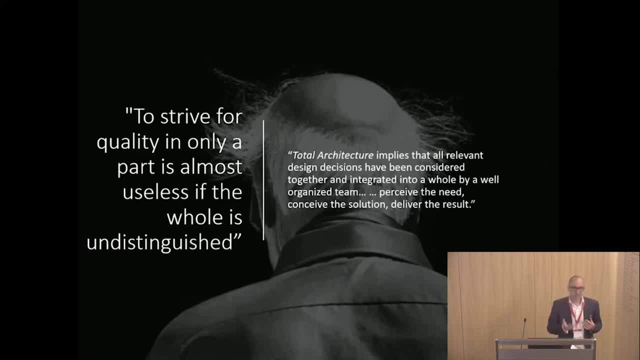 do, because it was it a real trust and respect for the different skills that people could bring to the project down to the people, our kind of knitting and sewing these nets without them in understanding how to put it together. if this couldn't be achieved, I think the quality of the documentation and that that we knew worked from a 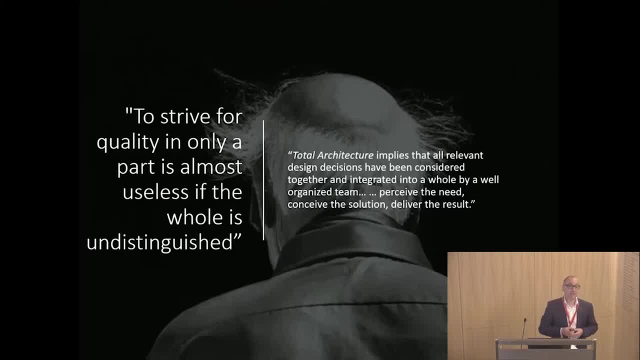 structural point of view, but the makers could read it from the making point of. I think the quality of that that spoke to both our needs was important and I think the quality of the outcome speaks for itself. so that's a. that was a kind of a where new materials and we have to. 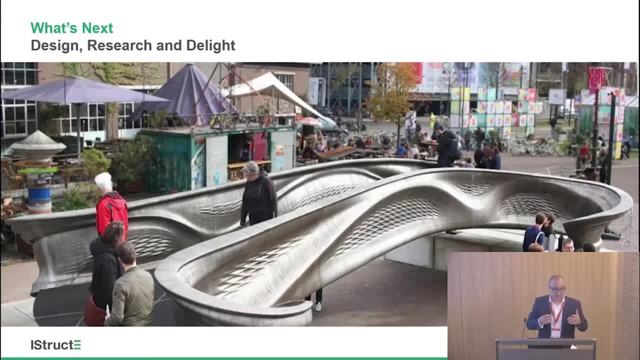 there's a probably a much longer talk about the research we had to do into understanding that the the allowable stresses within the ropes, the synthetic ropes, the natural fiber ropes and everything else. But there that was a materials, research, understanding, fabrication with a digital overlay. So it's a lot of the themes of the conference all coming together in one particular project. 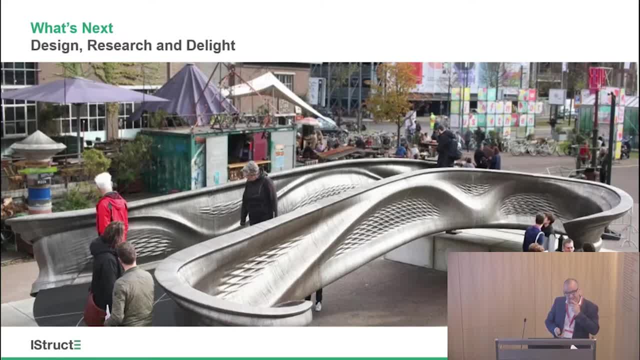 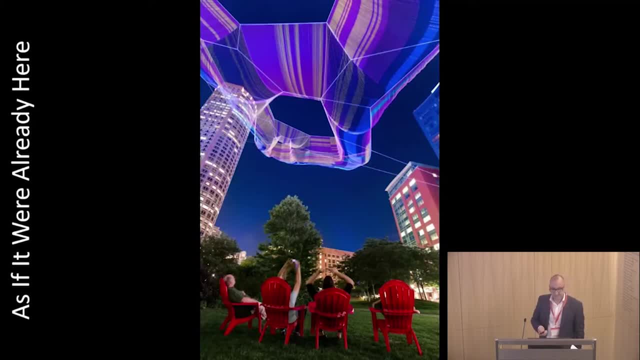 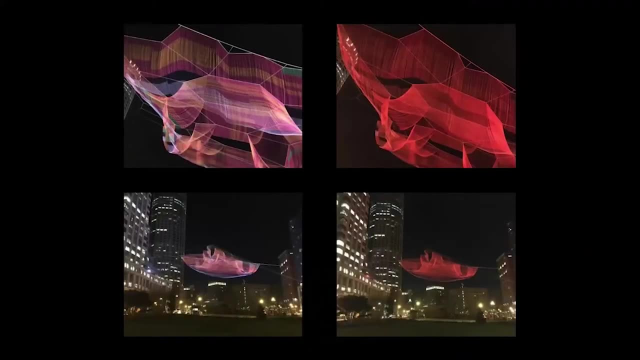 but now I want to talk about what's next- and I call it design, research and delight- and The work that we did on that particular project with with Janice. that has since developed into bigger, larger scale, Similar sort of sculptures. This is one in Boston over a huge park. 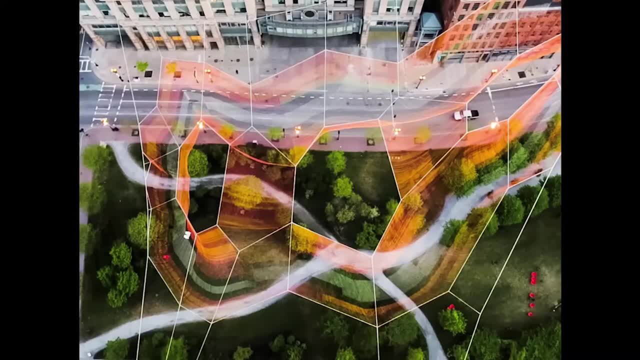 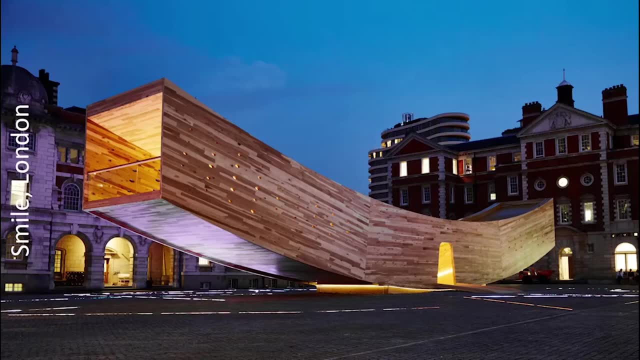 Creating quite a spectacular piece of public art that people can enjoy. this is a project that one of my colleagues in our did quite recently- and you might have seen it at the The architectural festival in London a couple years ago- called a smile. What I was interested about this is a couple of things. one is it's it's CLT, which is a material. 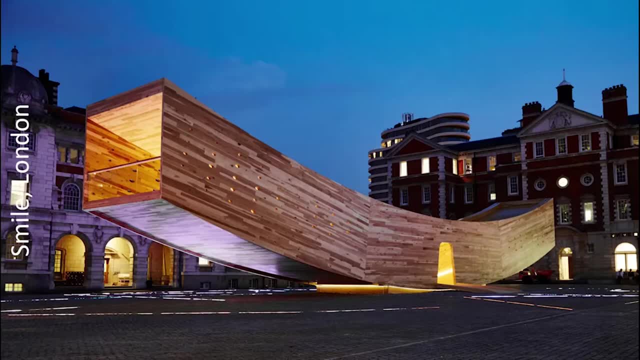 I think we need to explore. but actually it's. it's tulip wood and Actually this is an extension of the collaboration and the research that we did with the American Hardwood Council back on Portcullis house back in the early 2000s and the research 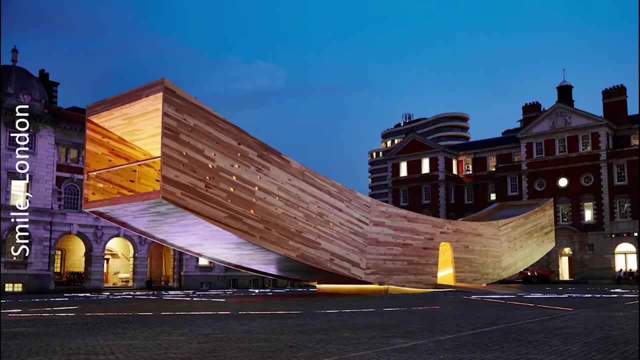 For the tulip wood was an extension of that. So it's a 15 to 20 year kind of research Collaboration together. So these collaborations between practitioners, academics, researchers, whatever might be, I think is really important if we're to drive Forward new materials, new ways of looking at materials and really understanding their behavior. I 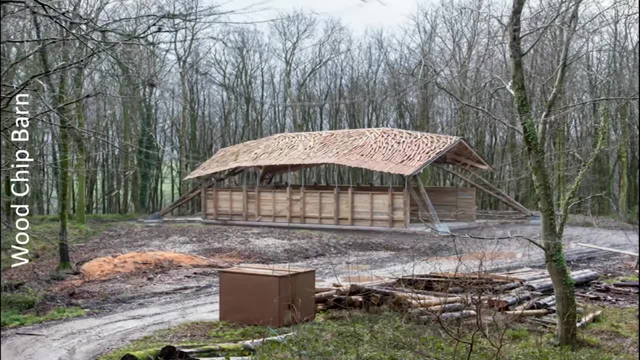 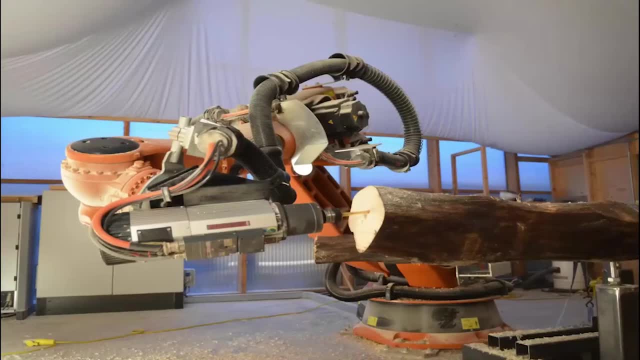 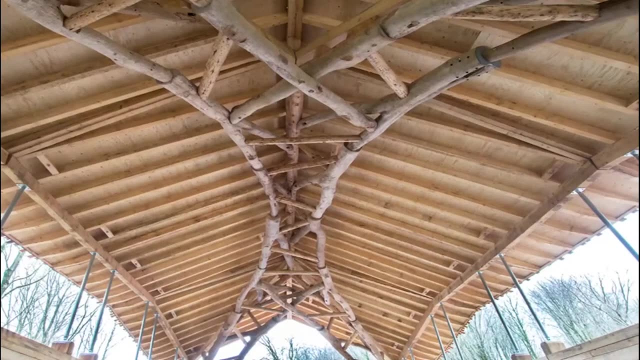 Think as well this one. I just think it's fun piece of a piece of architecture and design done by the Team. and what's really fun about this is they got this Chainsaw on steroids that just kind of cuts the hell out of these trees. But what I found really kind of interesting about it as well was that you know, sometimes we overlook 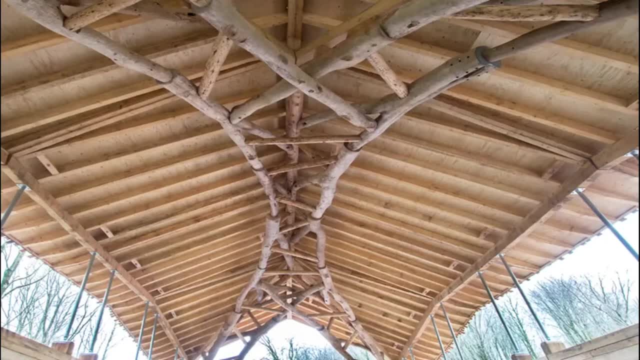 Valid pieces of structure, valid materials that can be used in a structural thing because they might look like normal. But what is normal? So the structural stuff here is done from basically Trees, branches of trees. We did that hundreds and hundreds of years ago, but along the way we said: no, everything has to be bright. 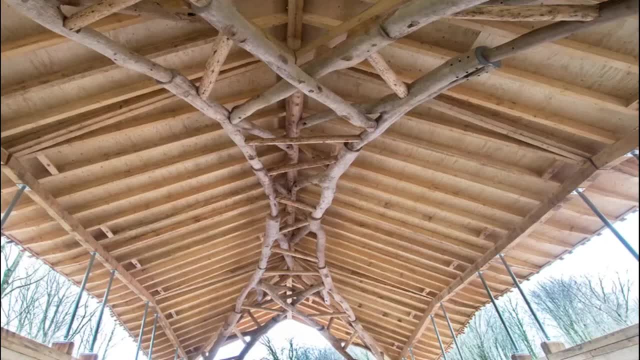 shiny and new. we've left some of the stuff behind and I think there's a place for some of this and I think we shouldn't. We need to put aside perhaps some of our biases and prejudices when we look at materials and rethink them and how we can use. 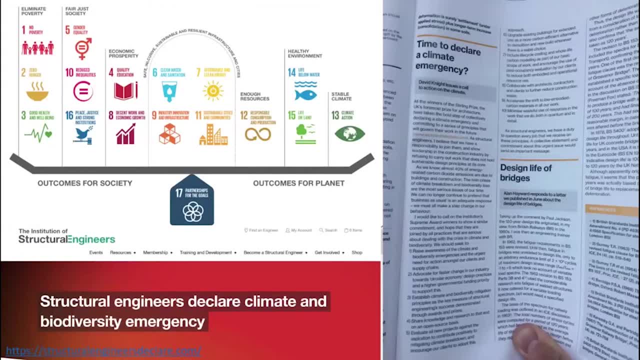 them appropriately. But actually I think there's a more serious reason why we need to continue our research Into material and alternative ways of doing things, and you- you all have seen, I'm sure, the UN SDGs, Which is important in terms of the outcomes for a panel- what we need to do for society and make a for a sustainable future. 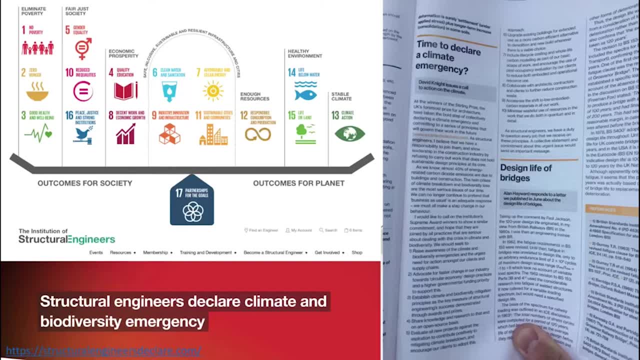 martin earlier on to talked about the declaration of the structural engineers made about climate and biodiversity emergency. that is real, it's happening now and we have we're running out of time to do something about it. and then two weeks ago in the um, the structural engineer, the journal of the ice- 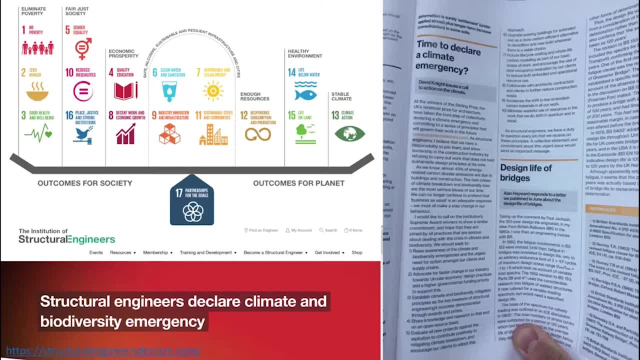 directory there's this letter by david knight saying it's time to do something about the climate emergency that we live in and actually if you look at the declaration i think it's really exciting and you might say it's an emergency. why are you so excited about it? but again, it's. 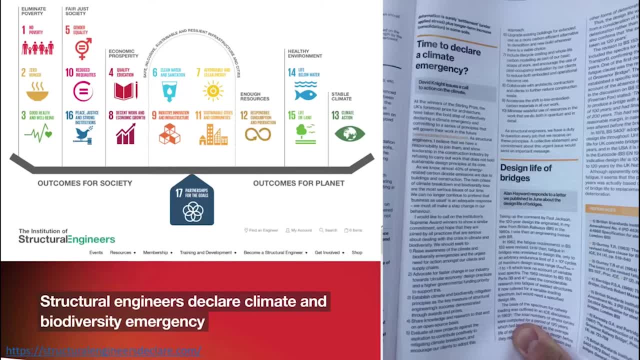 an opportunity for us as structural engineers, designers, researchers, practitioners, to make a difference in the world that we live in. and if you read i, i would urge you to read the um, the declaration, and the things that we said we're going to do. there's a place in that for 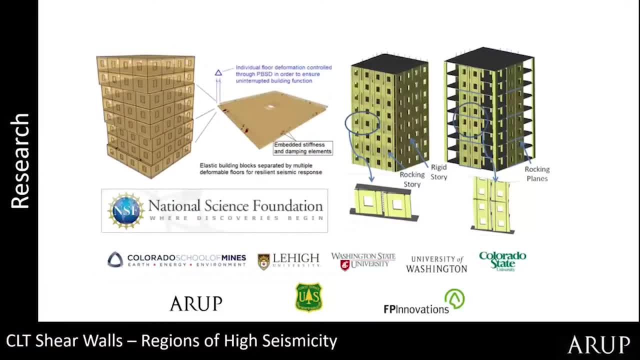 every single one of us to make a difference. so let's go do it and that, that research, i think you know we, um, this is some work i did when i was, when i was working in the states, and this is about clt, shear walls, you know clt, and timber is seen as a, you know, a sustainable 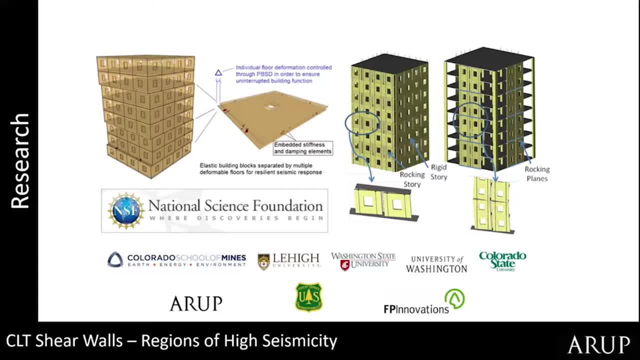 material, low carbon impact, but we don't know enough about it, especially in regions of high seismicity. so we did a lot of work on clt shear walls. but what i find interesting about this is not just the research itself, but the people that were involved. it really does take a village. 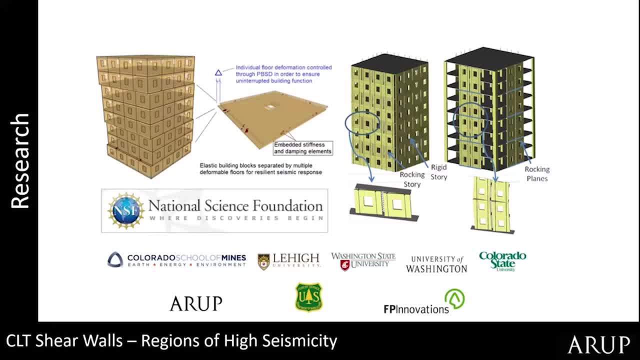 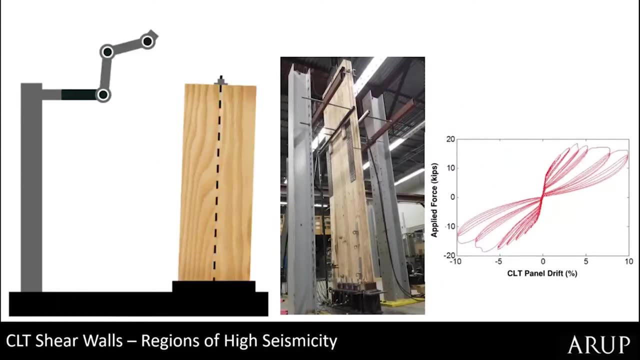 you know, no one can do it on their own. so this opening up, being open about collaboration and research and doing it together, it allows us to kind of um chart these uh uncharted territory to date and i think we need to do it. and you know this was absolutely leaning, cutting edge research that was done. 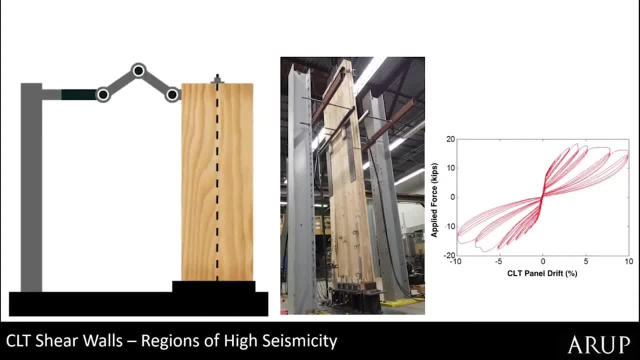 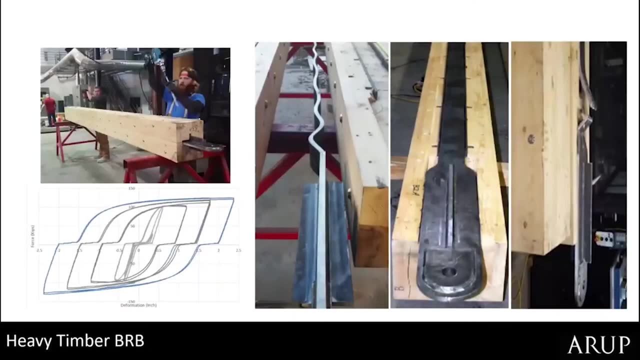 not that long ago and these technologies have now been used in buildings. so i think actually with digital tools and computation we can actually iterate much more quickly stuff that years ago might have taken us a lot longer to develop. so like from testing and research to implementation, that time span is a lot shorter now, and this is a similar piece. 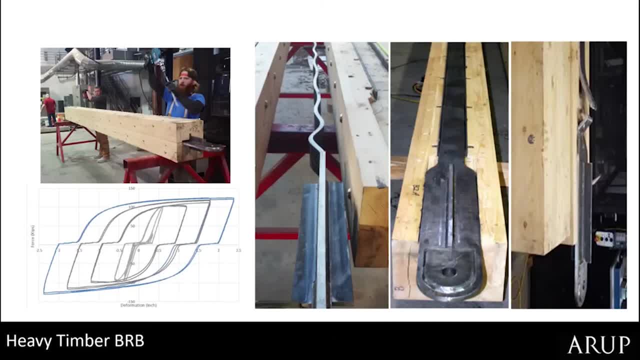 of research that we did on an alternative lateral system in regions of high seismicity, which is a bucking restrained brace. so here we are looking at a heavy timber brb, which is looking at technologies. brbs is a well-known technology in areas of high seismicity. 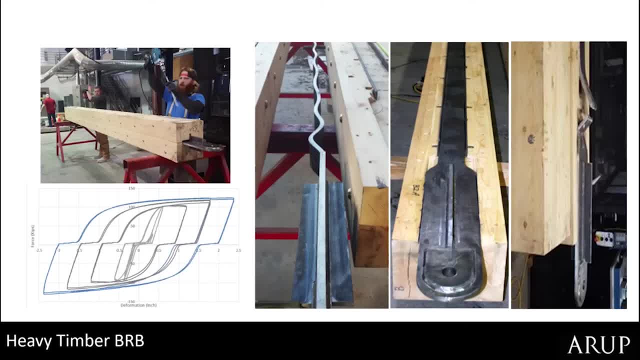 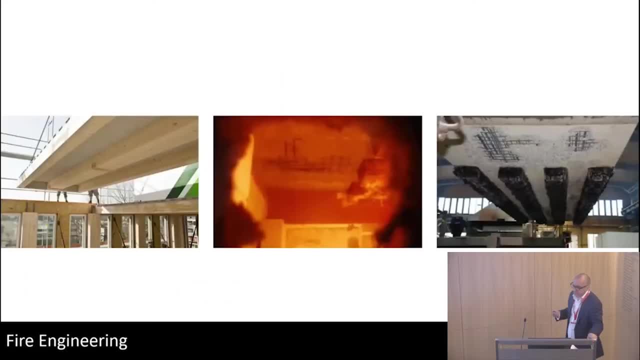 but not with um, with heavy timber. so we're bringing um two technologies together to see if it could lead us to a new way of doing things. and the research goes on. there's fire engineering and acoustic engineering that need to be done if we're to look at timber as a viable material. 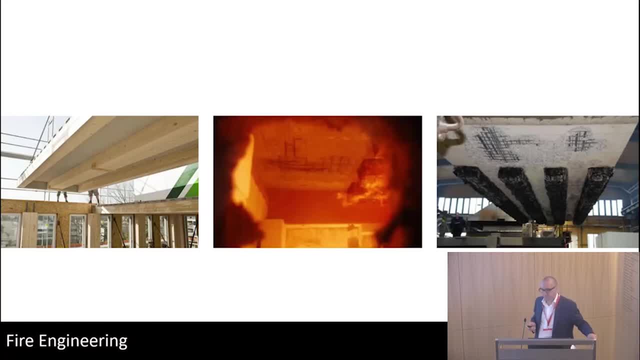 but together we can do it. this piece of research was funded by the united states department of agriculture because they were trying to create business in a new economy for the foresters by promoting timber as a viable construction material. the fellow was sustainable. they knew that to be viable they needed to address all these things. so there's good social and economic reasons. 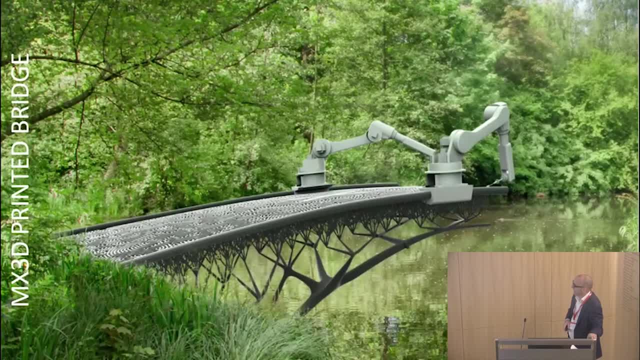 for doing these things as well. and then, you know, i look around arab and i continue to be inspired by some of the amazing people that we've got. so this is a friend of mine, matthew vola, from amsterdam office that did this amazing project, which was he was exploring with mx3d, the 3d printing of steel. 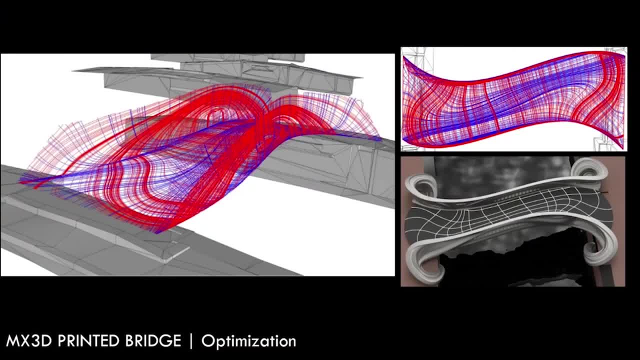 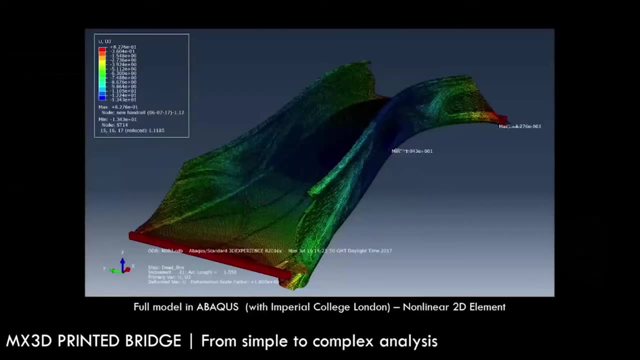 bridges, and again, this is some of the analysis that was done. but again, computers and the software that we have today was to optimize these things very, very to a final degree and just putting material where we need it, and it does the work. but that wasn't done in isolation. this 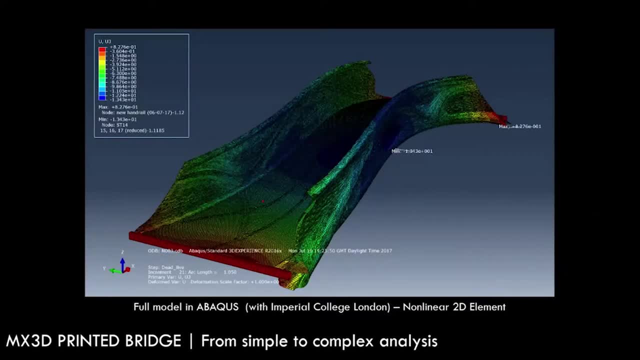 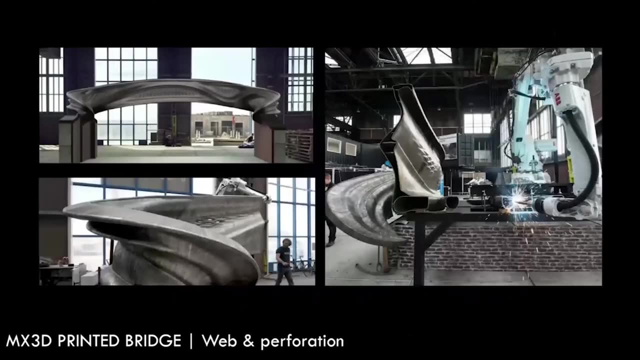 some of this analysis was done jointly with imperial college out of london. so our research crosses the boundaries and that will continue to happen, regardless of what happens on october 31st. and this is it, uh, the final piece. now let's see if this piece works. 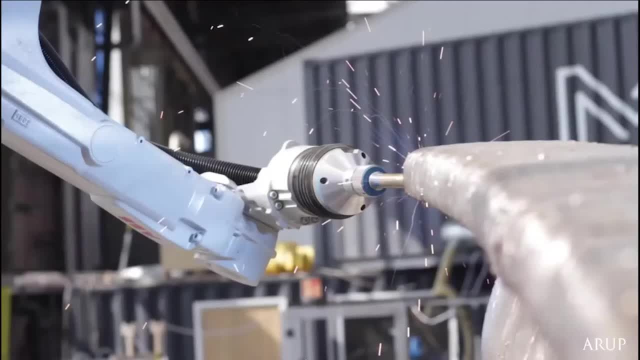 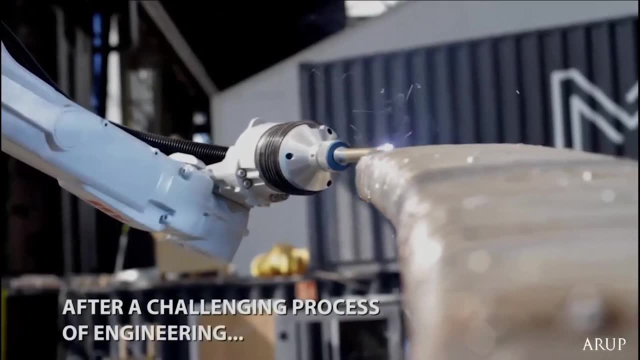 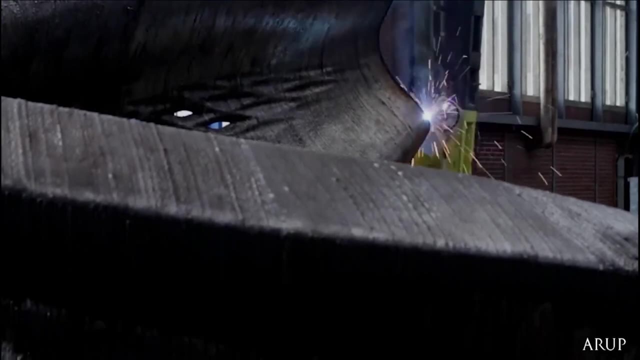 i think this is uh, let's see. so this is the actual process. but you know, these things look easy, but the stuff that behind all this is huge. i mean, there was unknown material properties. when you're printing 3d material and you have to figure out how do you deal with geometric inaccuracies and imperfections in this. 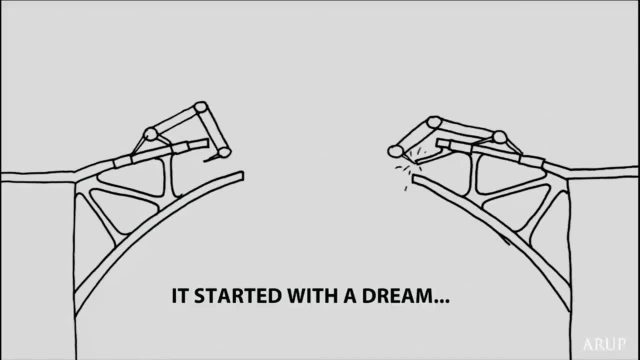 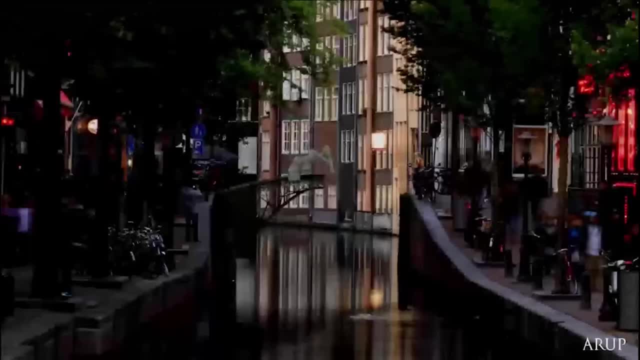 sort of environment in a 3d printed metal. what is the microstructure behavior of that steel material? what are the residual stresses and how does it impact your design? how do you deal with welding defects? so, but together we can solve all these things and create things that are. 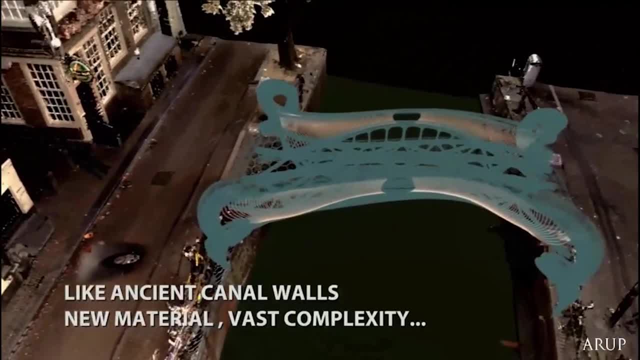 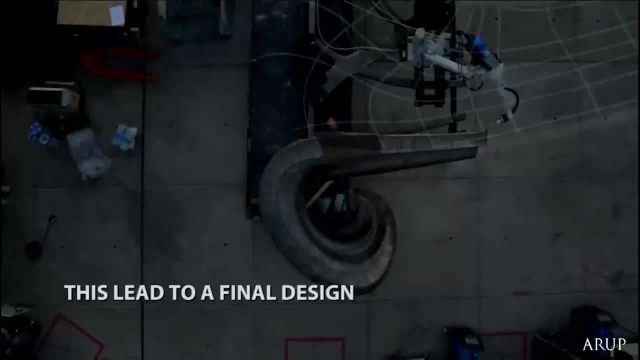 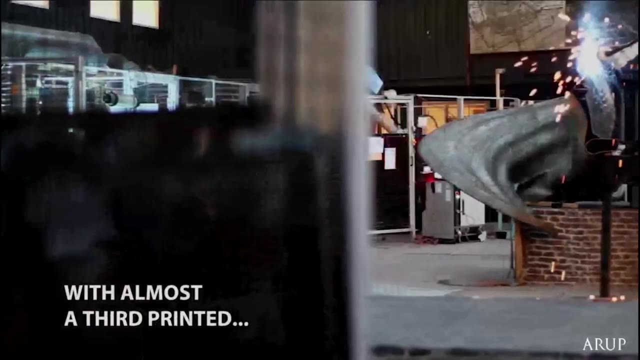 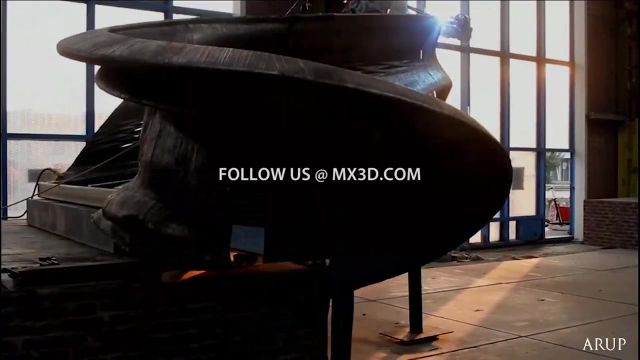 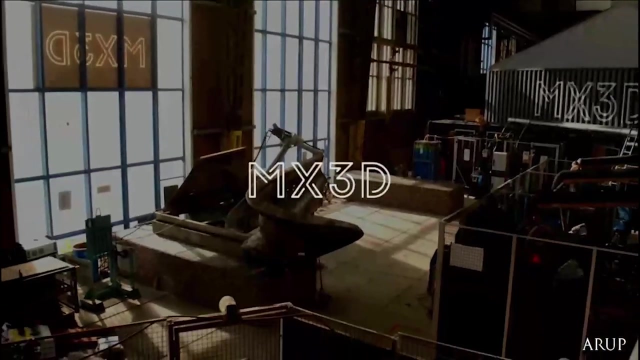 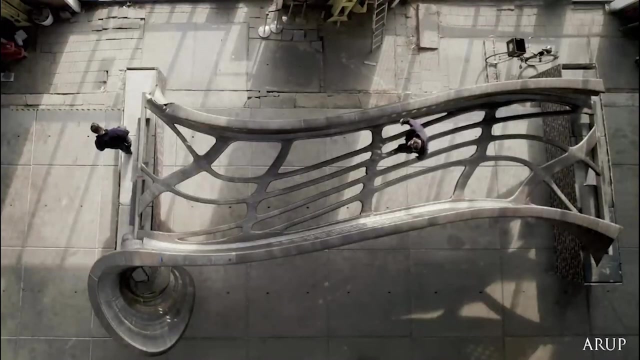 quite beautiful, quite stunning, and allow us to progress our industry and move it forward. so quite beautiful. sorry i should you know they. i cut the. sorry i should you know they. i cut the. that off too soon, but there was about a half a dozen people listed there. the 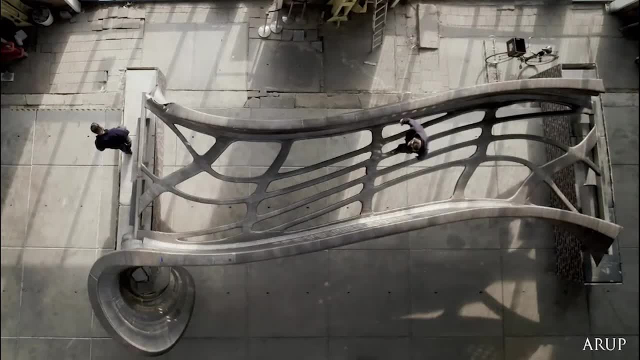 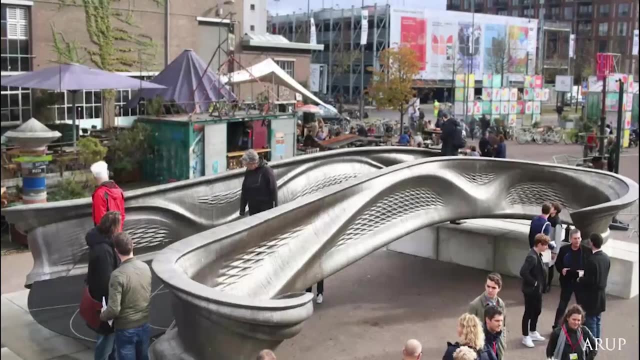 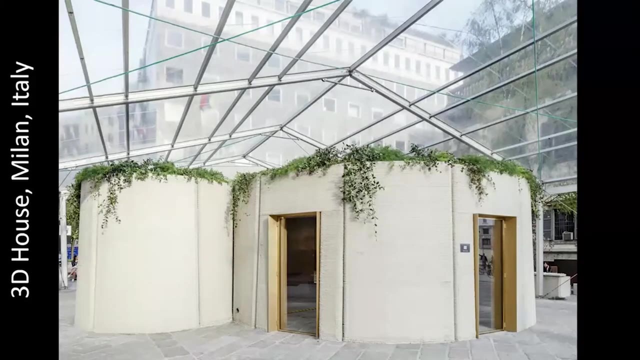 collaborators and that. so, again, it does take a village to chart new waters, but it's worth doing so. this is the finished piece, and that's the finished piece in place. absolutely beautiful, but not to be outdone. one of my friends in Milan, Lucas de Ville, looked at printing concrete, so this is a 3d house that was printed in. 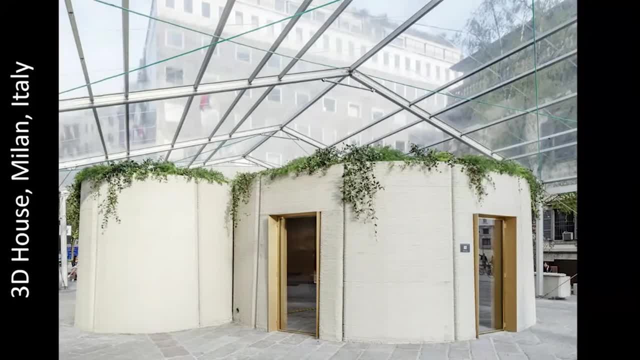 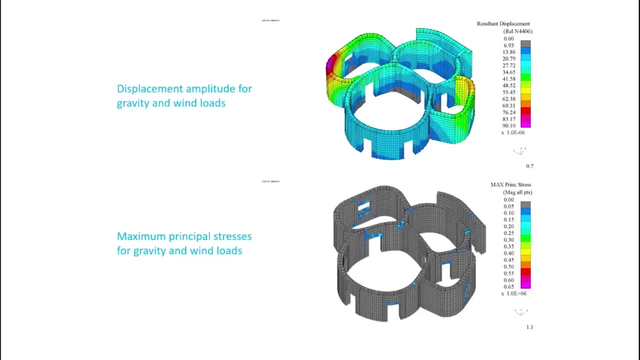 Milan for an architectural exhibition, and I'll look at some of the details in the moment, but each there's 35 concrete modules that make up this house, and each of the modules took about 60 minutes to 3d print, which is pretty impressive, and then assembled together to create the house. we did a lot of a, you know it's. 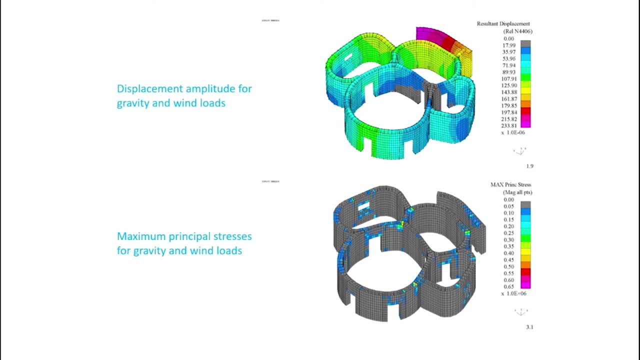 concrete. it's unreinforced concrete, so there was, you know, approaching concrete in a different way, and how it behaves and performs is. it took a little bit of thinking about how it's built. what the 3d printing process has on how the the material cures over time was things that 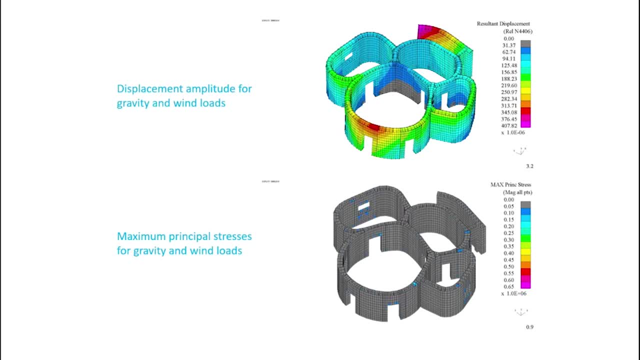 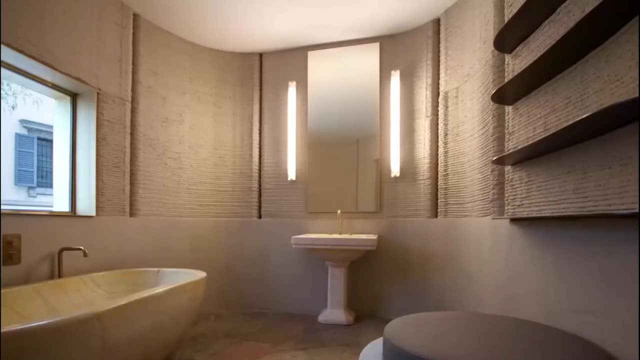 were unknown territory, so we had to figure all that out. so there is a place. you know, as engineers, there's a lot for us to do. computational tools allow us to iterate through that a lot more quickly. and this is what it looks like in the inside: quite beautiful, and this is. 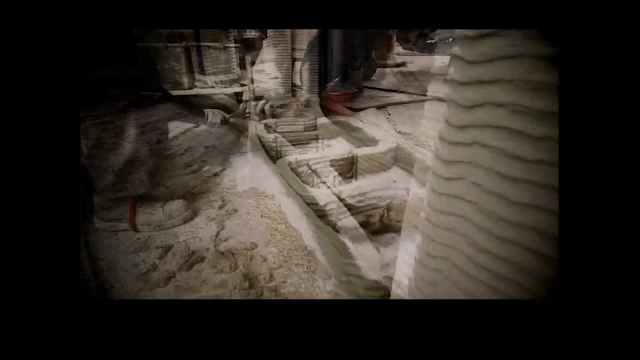 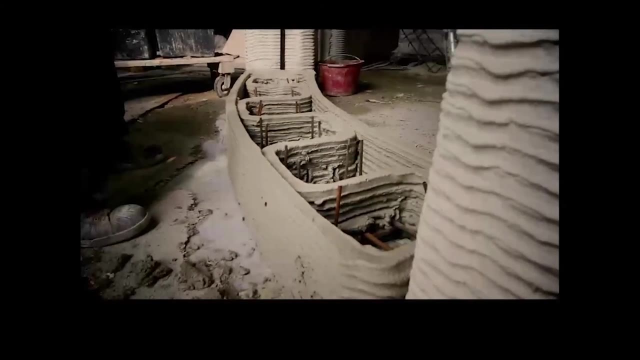 really, what I want to show you is this is a really unique piece of art that I started to do in 2009, and it's very interesting to see the kind of decoration that you can see on the wall, and it's a little bit of the same. 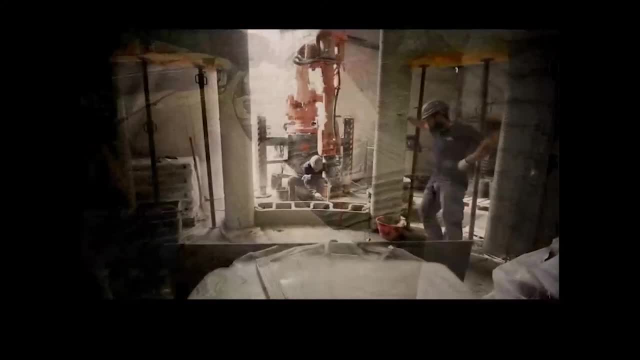 detail, as in the woodwork that I showed you earlier. it's a little bit of a different style and I can tell you that the details of this piece are very unique. it's a really unique, and I think that's one of the reasons why I wanted. 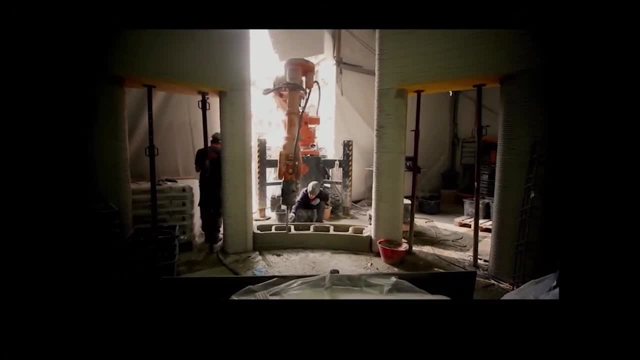 to go back and do this is because I've been working with a lot of these people and I've been working with them for a long time, and I wanted to do a project that was not just a project, but I wanted to show them the work that they 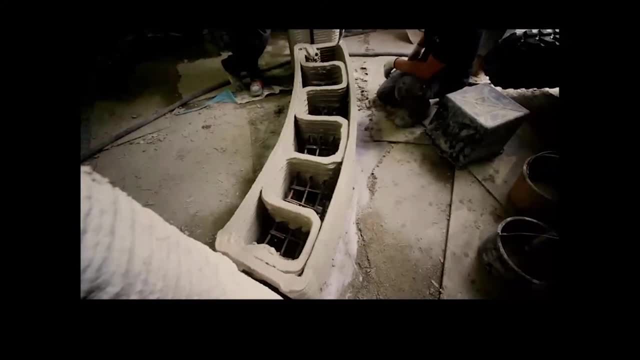 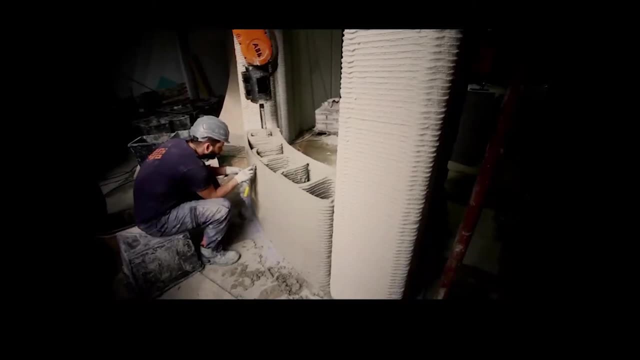 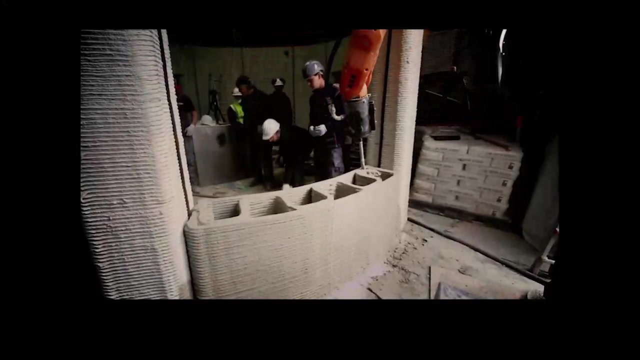 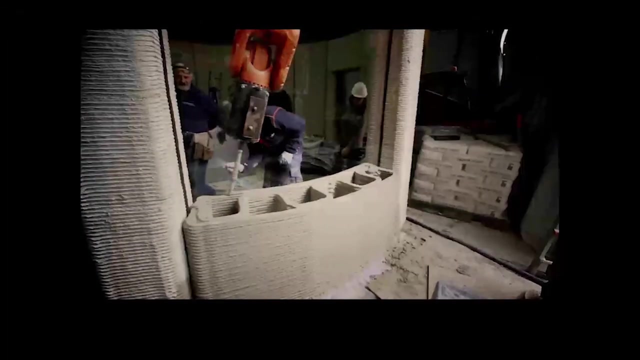 What I find interesting about this is: you know it's a 3D automated printing process, but there's still a man and machine sort of engagement. You know, if you look at the guy beside the machine, there's still that bit of handcraft. 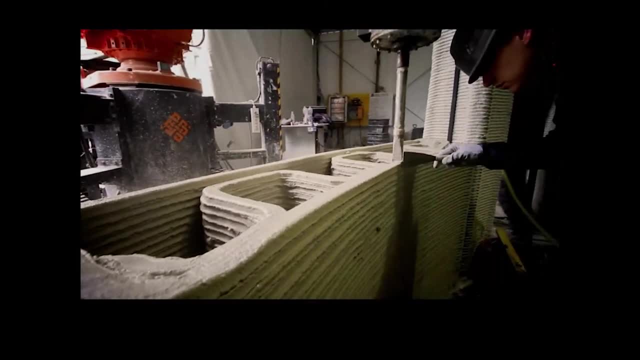 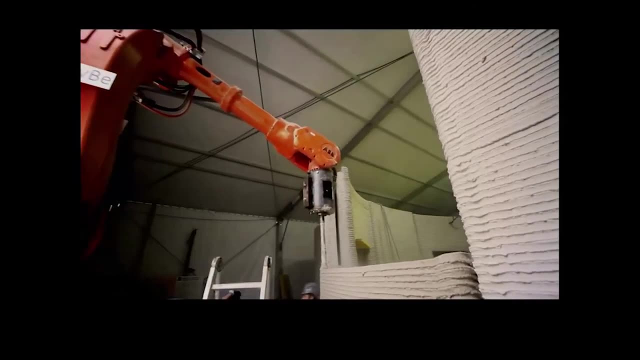 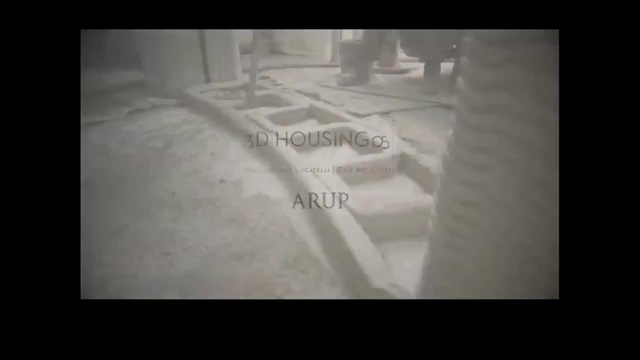 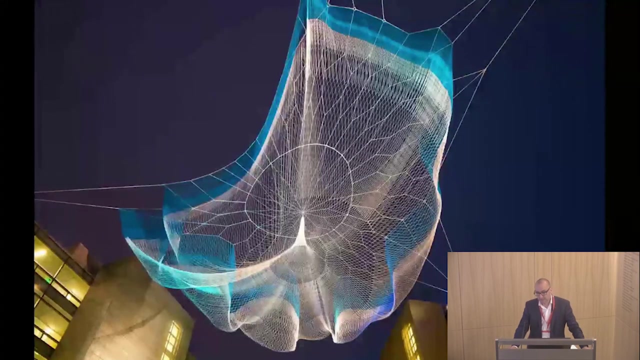 that's going into making this automated process. Okay, so again, a lot of people have helped to achieve that. You know, 10 years ago this wouldn't really have been possible, but now it is, and technology is changing so quickly. 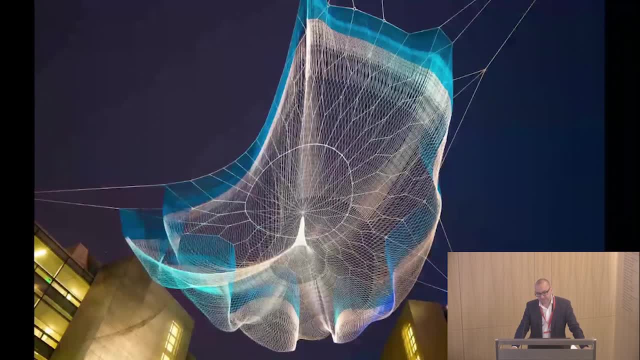 But you know, it is a critical time for the planet and I think, as engineers and designers, we have a huge responsibility, But also a huge opportunity to make a difference. I think there is significant work for us to do and, as an industry, I think we need to. 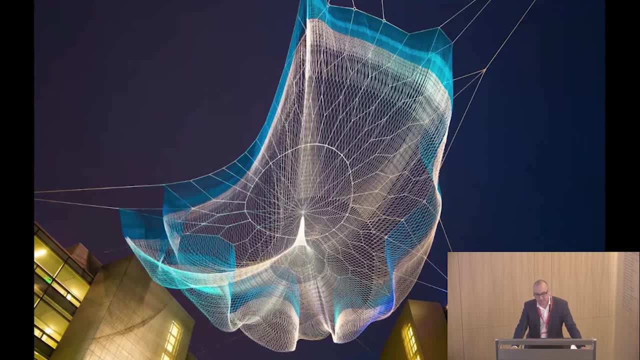 harness our collective skills, our expertise and our intellect to create structural engineering outcomes that have a more positive impact on the world around us. I think, with an improved understanding of materials- old and new materials- coupled with digital technologies, automation, machine learning, I think we're at a fairly unique 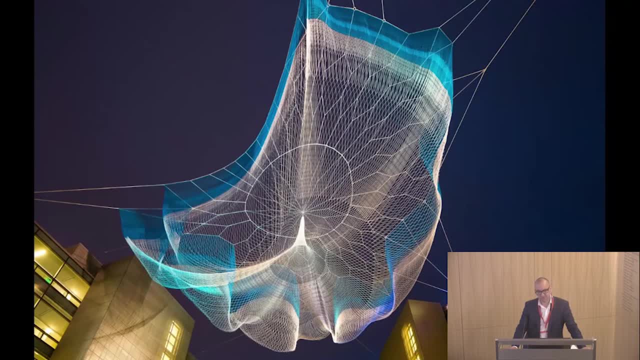 point in history, But I think that gives us the opportunity to make a difference And solve the problems that face the planet today. I think optimization and rapid prototyping, both real and virtual, allow us to explore and understand the impact of our designs in a way that we have not been able to do before. 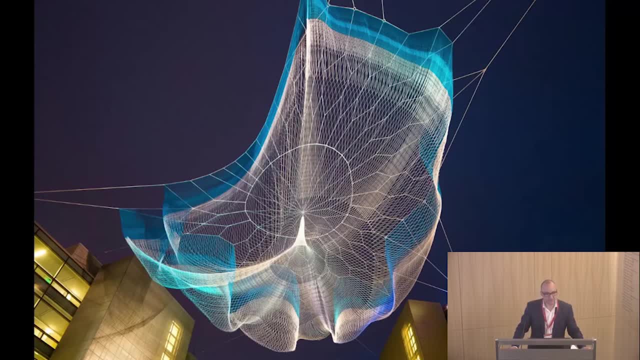 So I urge you to take the opportunity to do something different: Explore, create, solve the problems of the planet, because it's in our interest to do so, but it's in our gift because we have the knowledge and expertise I think open up your minds and your hearts.